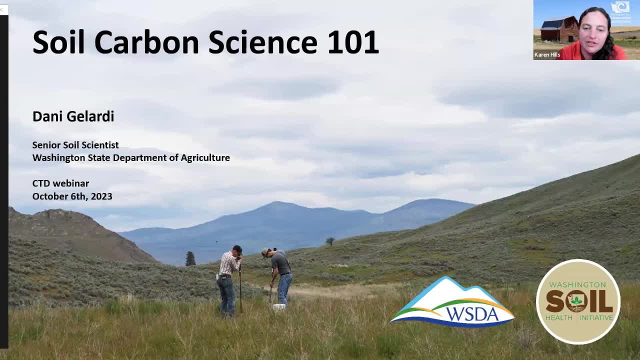 She received her PhD in manufacturing and engineering and she's also an adjunct faculty at Washington State in soils and biogeochemistry from the University of California Davis, And we're just really happy to have her here today. So, without further ado, I'll hand it over to you. 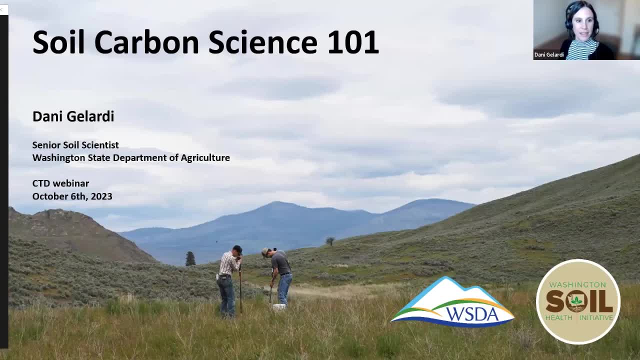 Danny. Thanks Karen, Can you hear me okay? Awesome, Hi everyone. Thanks Karen for the introduction and Jan for having me here today. I am very excited to talk about probably my favorite topic to people who actually want to talk about it. Usually it's just me kind of clearing a room at. 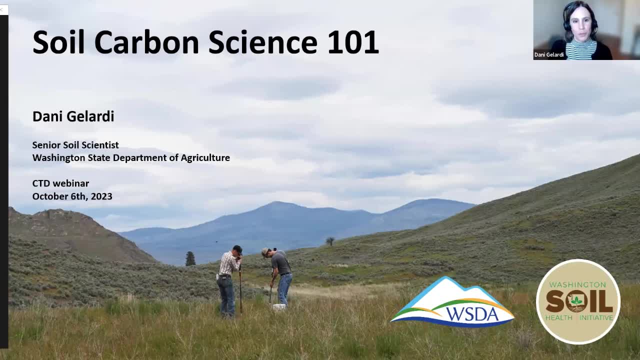 a office, but I'm really excited to talk about it. So I'm going to start with you. Danny, cocktail party, So welcome. Let us talk about soil carbon. If you work in agriculture or in climate, or if you've been paying attention to the news at all, you've probably been hearing about. 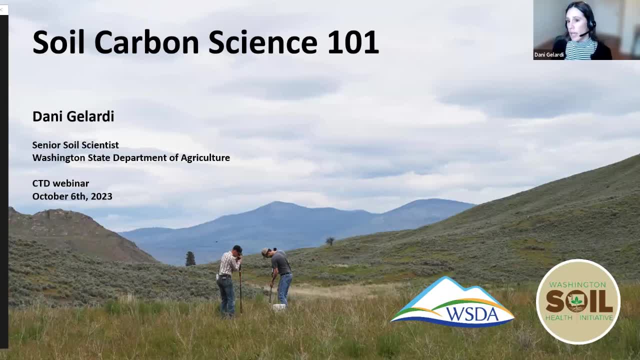 carbon, and specifically soil carbon. So today I hope to provide just some of the basics of soil carbon science so that we can all better interpret what's happening in the popular press and better make decisions for our farms and our farm stakeholders that are rooted in science. 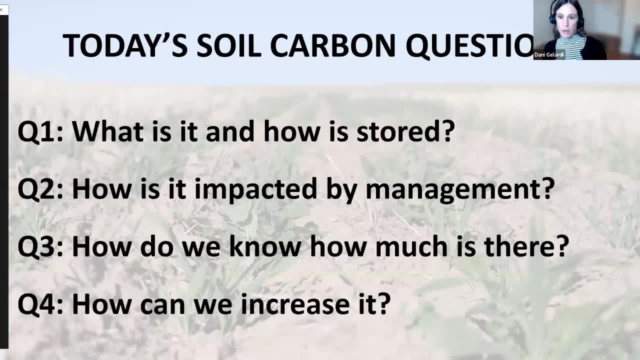 So it's a big topic to cover in just a short webinar, but I hope to at least begin to address some of these questions. What is soil carbon and how is it stored? How is it impacted by management? How do we know how much is actually in there And, importantly, how can we increase it After each of 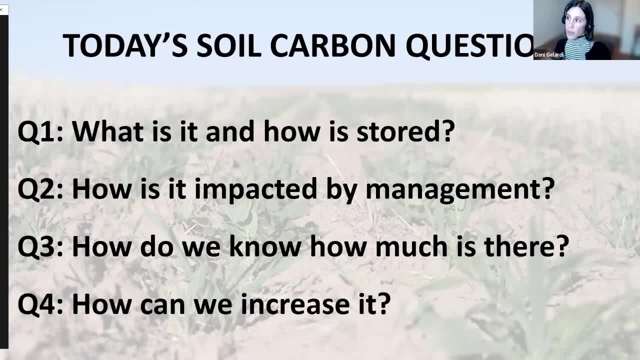 these sections, I'll pause and check in with you. So let's get started. I won't be able to see it while I talk, but there will be kind of a quick pause after each section and I'll see if you guys have any questions and try to answer them along the way. 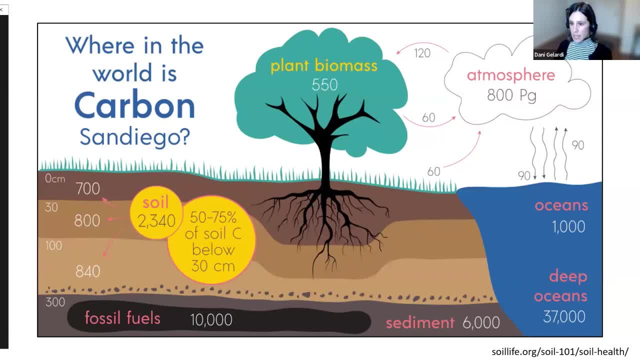 So where in the world is carbon? San Diego, A question I ask myself every day. Carbon gets a lot of attention, mostly because atmospheric concentrations are increasing. This, of course, makes big news quite regularly and kind of has an urgency to the carbon. 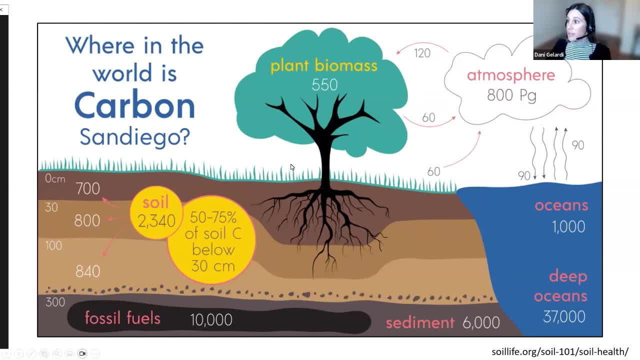 Discussion, And the carbon in plant biomass also gets a lot of attention, mostly because it's visible. We've known it's there for a long time. We can see it. It's fairly easy to estimate how much is there. But today we're here to talk about the invisible carbon sink that is beneath our 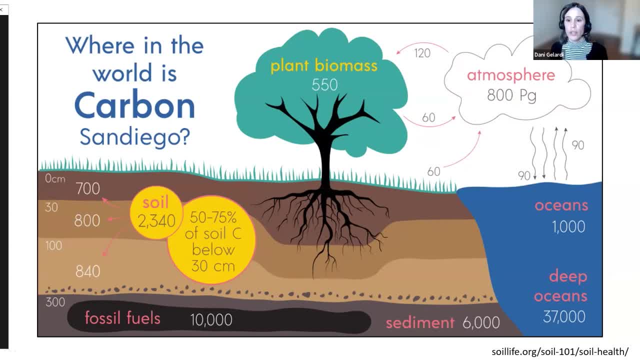 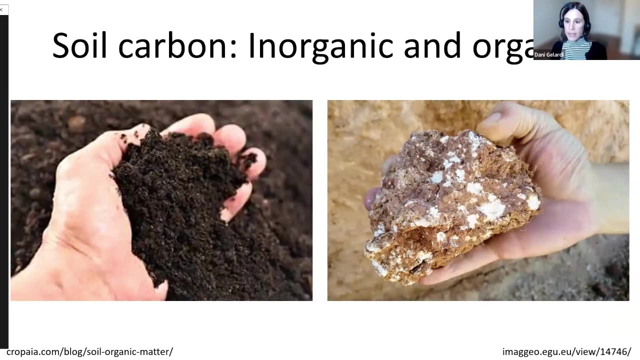 feet, which, importantly, is actually a larger carbon sink than the vegetative and the atmospheric carbon combined. So we're talking a massive terrestrial store of carbon. So let's get started In the soil. carbon exists in many, many different forms, But broadly, the kind of first split in 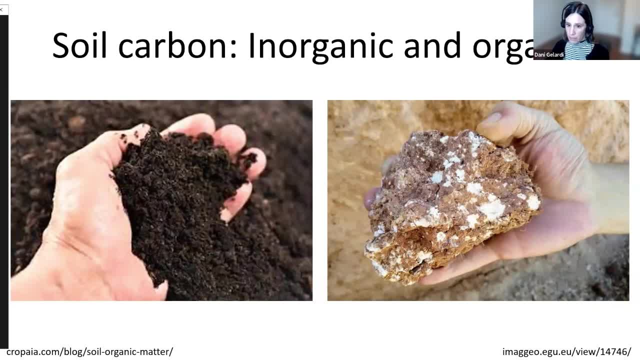 categories that we talk about is organic and inorganic forms. So here on the left we have soil, organic matter. This is the 1 to 5% of most soils that is not made up of minerals, air or water, but is instead made of animal and plant tissues in various stages of decomposition. So 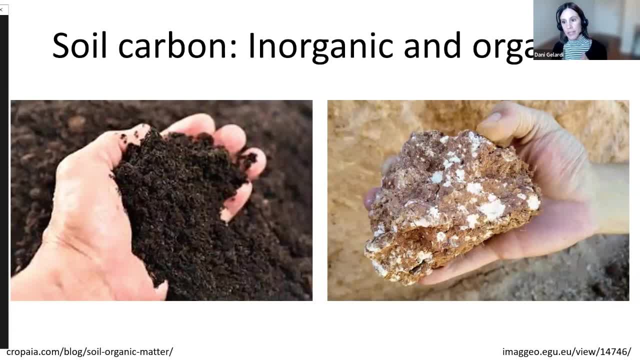 you'll often hear soil organic matter Or soil organic carbon used interchangeably SOM or SOC. It's not incorrect necessarily, but soil organic matter is roughly 58% soil organic carbon. The remaining portion of soil organic matter includes other essential plant nutrients like nitrogen, phosphorus, sulfur, as well as a lot. 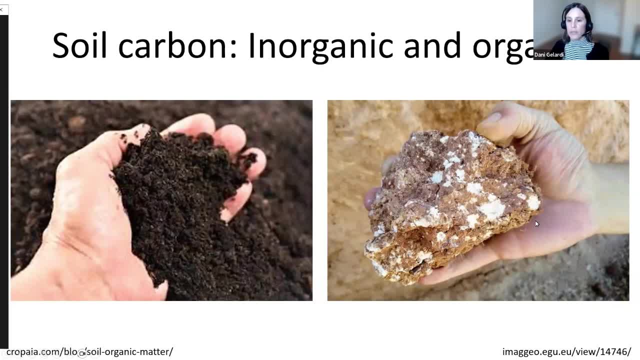 of hydrogen and oxygen. Here on the right we have soil inorganic carbon. This is primarily found as carbonates in arid environments. So if you're in eastern Washington, for example, you've probably come across a caliche layer or a sort of hard pan of calcium carbonate beneath the soil surface. 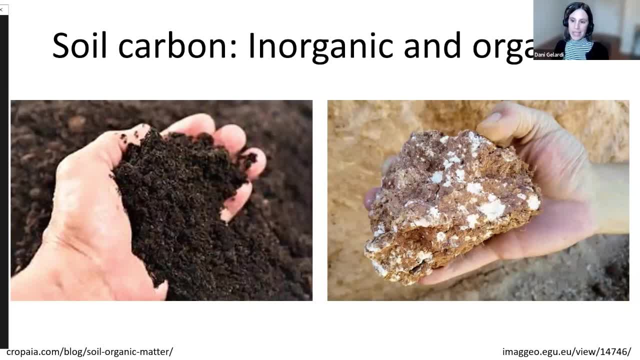 And this is actually rich in carbon. It's just inorganic carbon, And while carbonates are an important component of soil carbon, they're generally considered more difficult to increase via agricultural management, And so we don't talk about them as much. in the soil carbon or 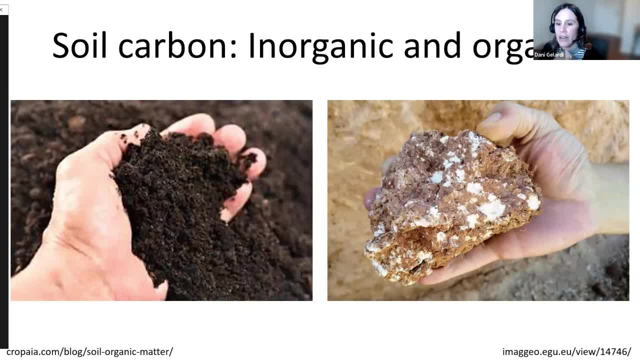 regenerative agriculture space, They're mostly just an arid environment. So if you're in an arid environment, they're usually just an arid environment And altogether they represent a smaller pool than the organic carbon here on the left. There are, however, some strategies to 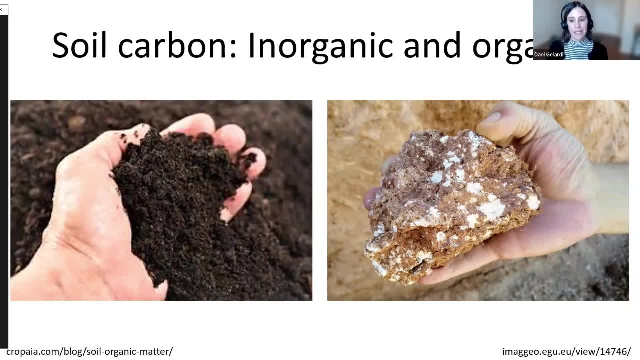 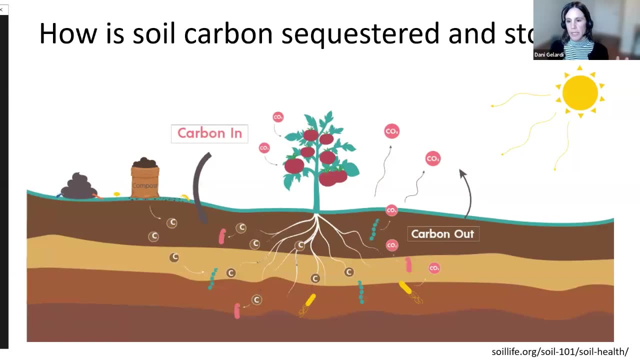 increase soil inorganic carbon. You may have heard of things like enhanced weathering or crushed basalt amendment. We won't talk that much about that today. We're going to really focus over here on the organic portion of soil carbon. So let's start by just some of the real basics. 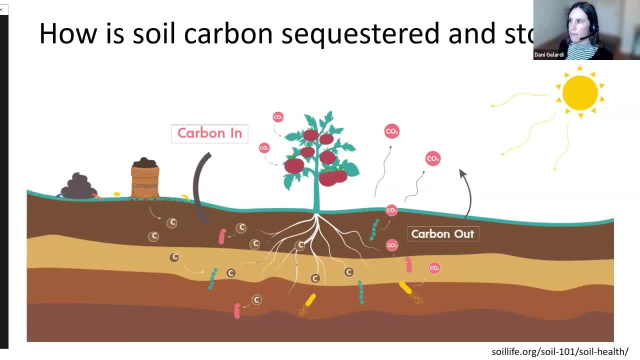 How does carbon get into the soil? And in the process, let's define a few. So plants use atmospheric carbon dioxide. during photosynthesis, They convert that gaseous carbon into sugars that are then stored in their vegetative bodies or exuded. 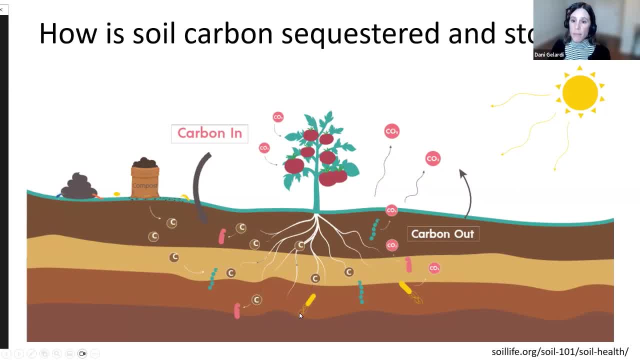 through their roots into the soil And then soil microbes use that vegetative carbon in dead plants, leaves, root exudates, along with dead micro and macro fauna, manure, compost, biochar and other organic materials as a substrate for metabolism and 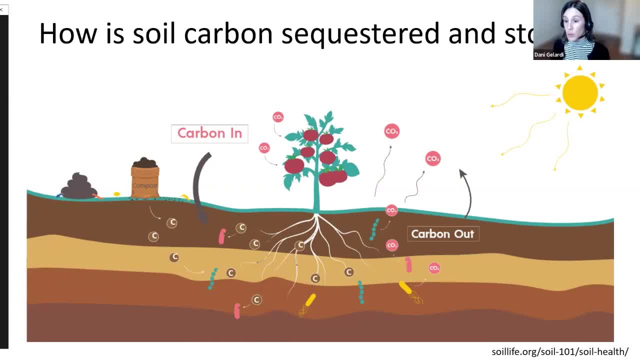 population growth. So just like humans need carbon-based food to survive, so do microbes, And in the process of microbes using that carbon, actually much of that carbon is then released back out into the atmosphere as CO2 and released into the atmosphere. So something like 3 to 33%. 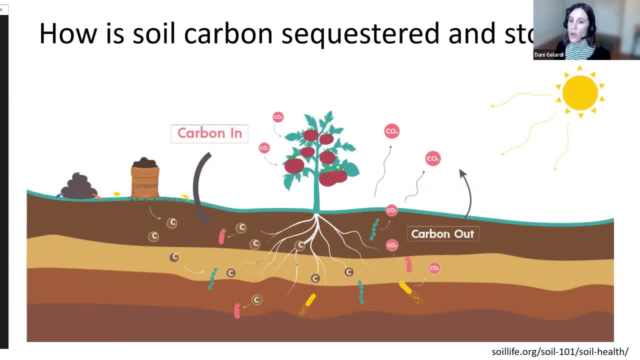 of carbon inputs is retained in soil, organic matter or in microbial bodies. So I just want to define a couple of terms that often get used interchangeably And, again, it's not incorrect, but there are some nuances that are important to think about when you're trying to interpret popular press stories or even policies. 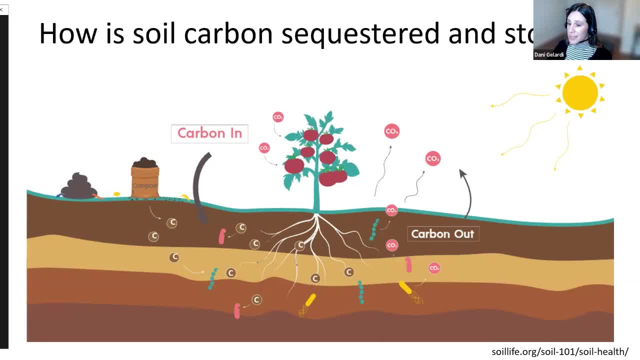 that are coming out. So the biophysical process that I just described, by which gaseous carbon is drawn down, processed by microbes and added to the soils, is called soil carbon sequestration. The amount of carbon sequestered minus the amount lost is called soil carbon storage. 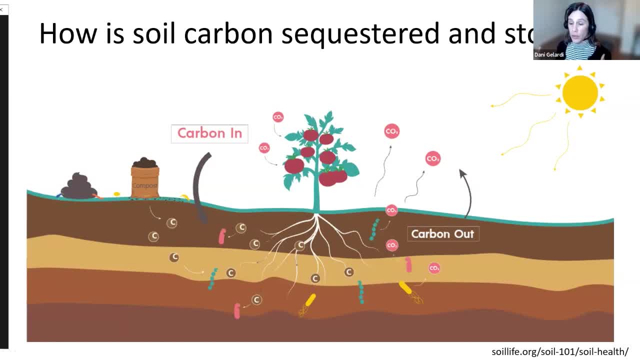 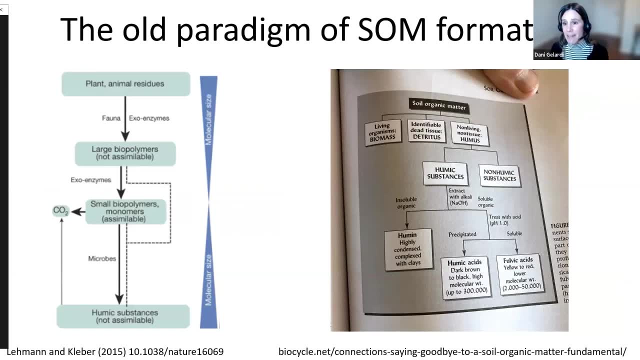 And, of course, it's storage that we are hoping to increase overall. So we want to sequester more and lose less. Over the years, our understanding of how soil organic matter forms has changed a lot. If you studied soil science at any point prior to the last decade, you may remember seeing these figures. 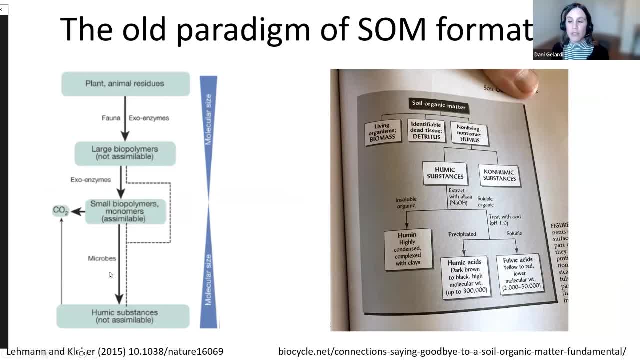 about a process called humification. This was an early notion based on an extraction method in the lab that assumed basically a humification process, And so we're going to talk about humification process. created recalcitrant or resistant to decomposition humic substances to make up the 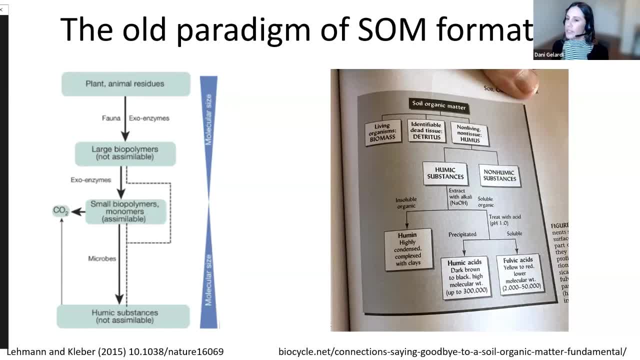 majority of soil humus. As research techniques have advanced, however, we found that a lot of these humic substances were mostly just an artifact of the harsh chemical extractions we were doing in the lab. So when they looked at actual naturally occurring soil organic matter, 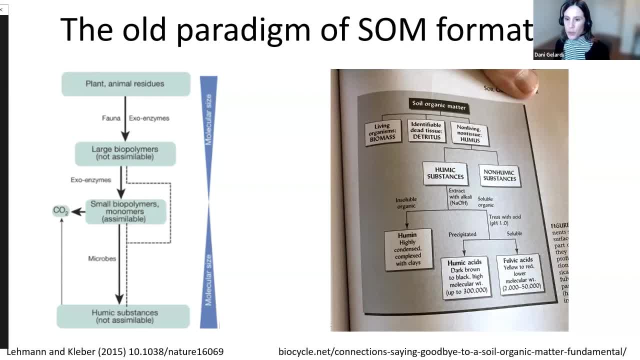 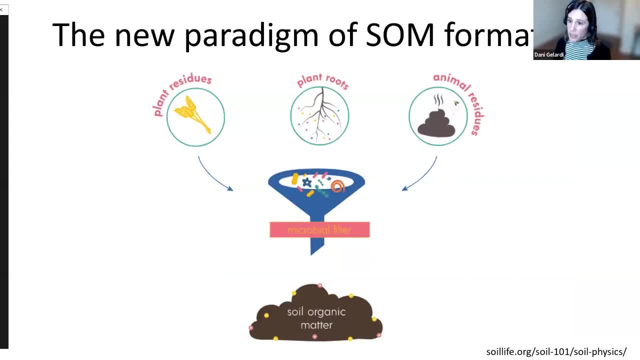 they found that those distinct humic, fulvic and human categories didn't really occur naturally in the soil. We now talk a lot less about humification, but instead talk about the microbial filter. This change in the soil organic matter paradigm brings soil microbes to the front in the formation of soil organic matter, And this is important. 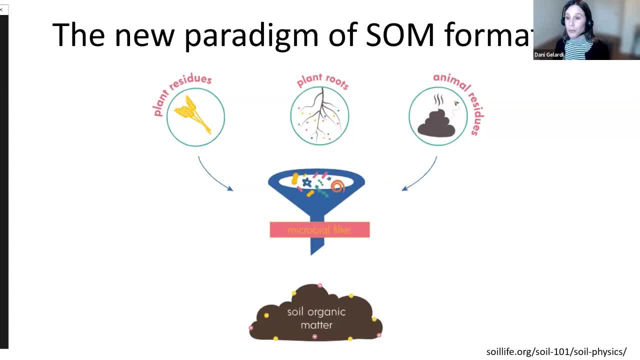 because a lot of people on this call are probably really excited about soil health, And part of what's so great about soil health is that we're finally talking about biology- And that's true also in soil organic matter- formation paradigms, Rather than just breaking down plant materials until what is left is soil organic matter. 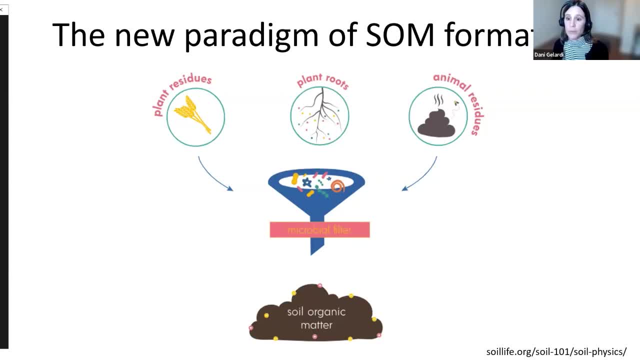 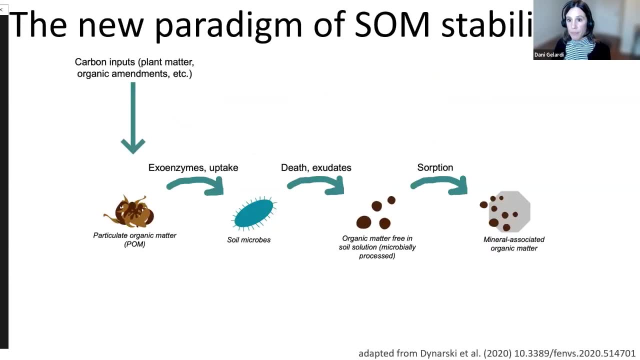 we now know that soil microbes are actually producing the compounds that become soil organic matter, And when they die their necromass also becomes soil organic matter. So here's a kind of flow chart for what that looks like. The carbon comes in, passes through. 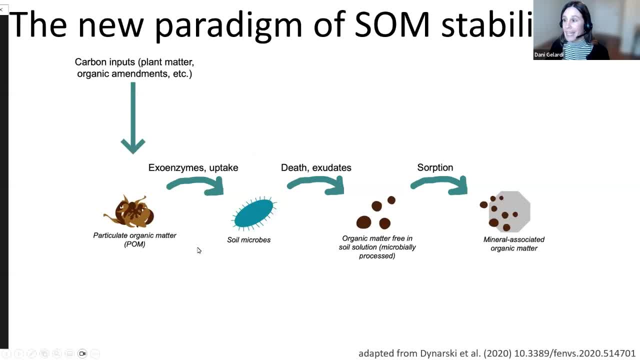 the microbial filter somewhere around this phase And ideally it makes it all the way to, as it is organic matter, very quickly. Now most people do know theって here. this kind of every specific venue for mineral composition- I'm going to call it- is once evaporation. 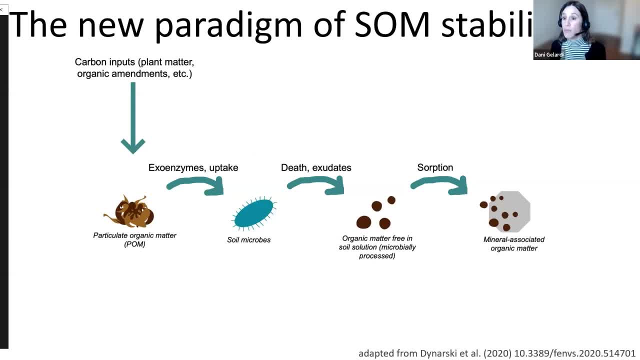 And the tufts usually start just coming up. And I'm going to say one. it goes from Starting out here. can you see where the the next set of Laws here- Yeah, I sentencees inerals. other mineral-associated organic matter does have its own loss pathways. Each of these phases has 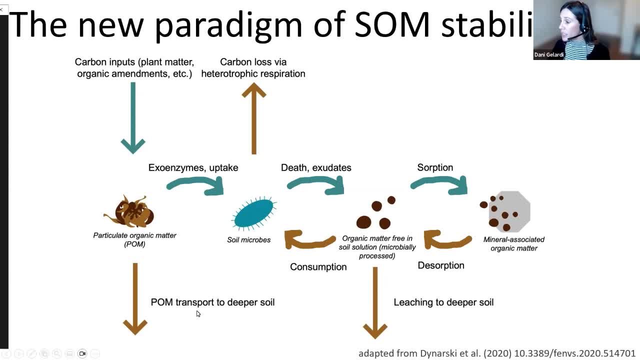 different potential to be lost, either through leaching or transporting deeper into the soil through respiration, microbial respiration and so on. So I show this to emphasize that soil is not just a sink or a source of carbon, but it's really a part of the carbon cycle, Another way to look at. 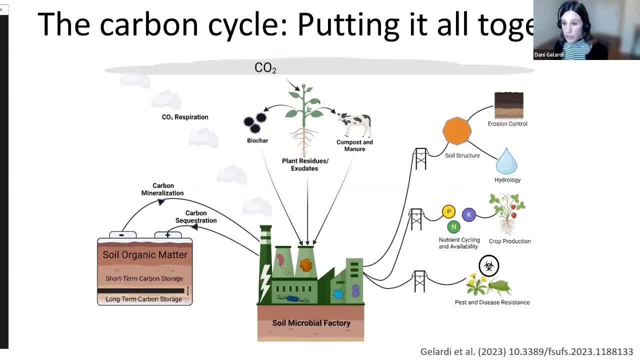 the carbon cycle is to think about soil microbes like a little factory that both charge and draw power from a soil organic matter battery. So the charging process like we've talked about is called soil carbon sequestration, And then mineralization is how microbes utilize soil. 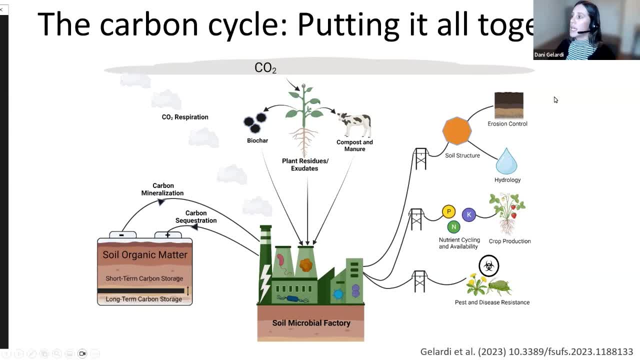 organic matter for various ecosystem services. Here we see ecosystem services that power a lot of what's important about agriculture: things like water supply, nutrient cycling, pest and disease suppression, of course, all of which are in the service of producing food to feed. 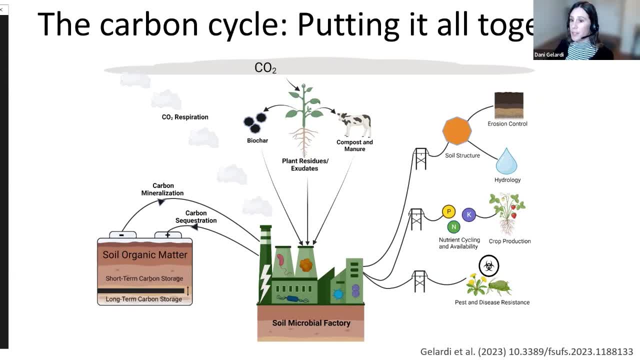 a growing population. But in order for these services to be provided, microbes have to use that soil, organic matter and in the process, release much of that carbon back as CO2.. It's not a bad thing. It's an inherent part of this carbon cycle and food production. 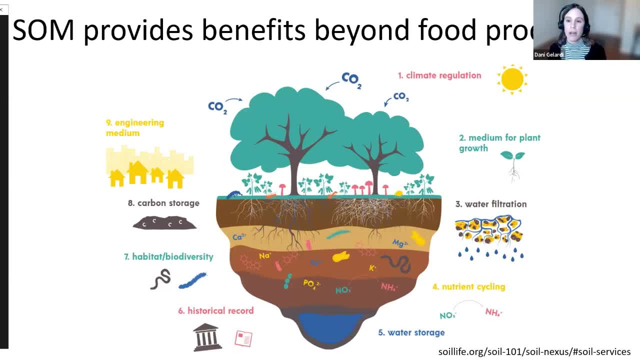 And, of course, agricultural services are not the only thing that soil organic matter provides. I think we talk a lot about agriculture in this space, but humans are not the only ones that benefit from soils and soil organic matter. They're an incredibly large sink for soil carbon. 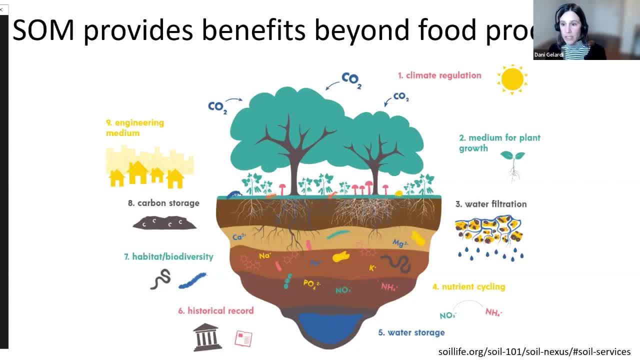 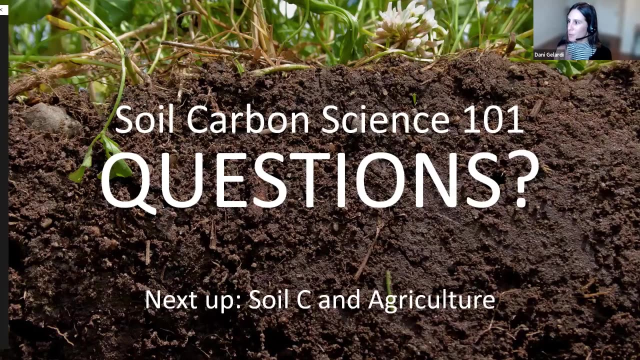 and therefore help us regulate climate and mitigate climate change. They're also incredibly important for water storage and filtration and for providing biodiversity habitat for macro and micro flora and fauna. Okay, that's kind of the quick and dirty way to look at it, But I think it's a great way to look at it. 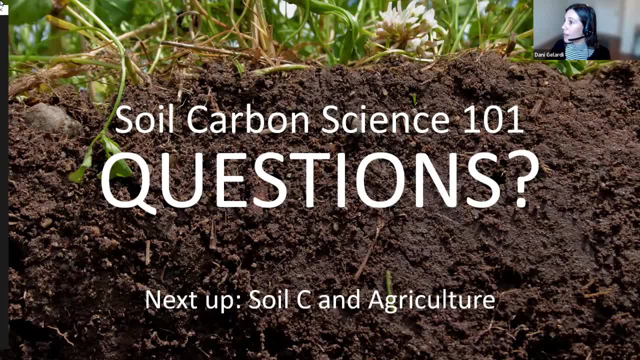 Soil: Carbon Science 101.. Next we're going to talk about how agricultural management impacts it, And I'm going to quickly check the chat And we have someone here from Nigeria. Welcome, I'm so happy you're here. I'll pause just for a few seconds and see if anyone wants to ask something. 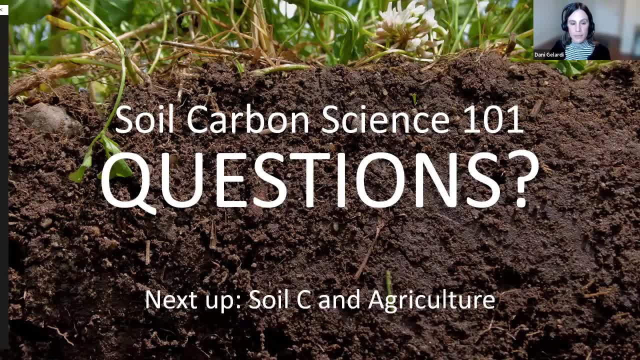 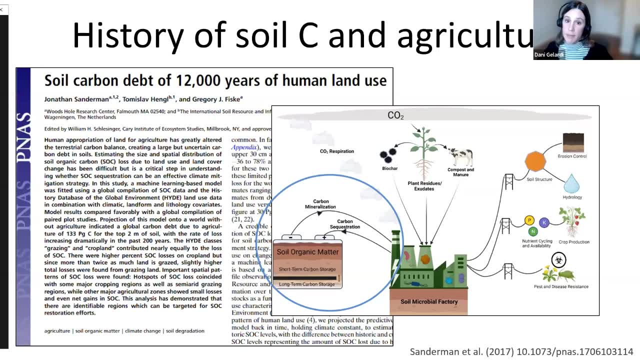 And if not, I will keep going. All right, There will also be time to ask questions at the end, if anyone has them. So let's talk about agricultural management. I think that's why a lot of people are here. Soils are indeed an important soil carbon store, And there is great evidence that shows that. 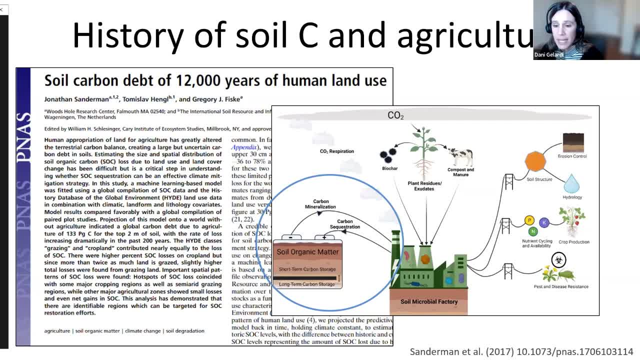 naturally low carbon soils can actually sustain increased storage as a result of agricultural management. However, as I described, agriculture necessarily and inherently exploits soil carbon for crop production. In fact, this paper here shows that over time, humans have incurred a debt of 133 pettigrams of carbon from soils worldwide. 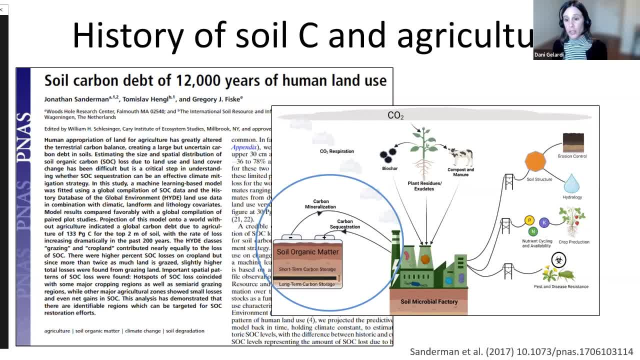 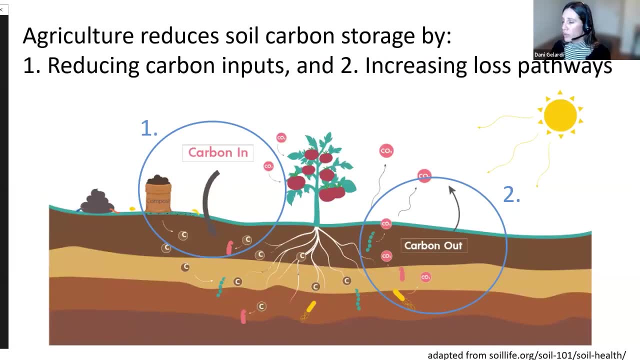 with hotspots unsurprisingly associated with major cropping regions and degraded grazing lands. This means that a not insubstantial amount of carbon in the atmosphere used to be in the soil and was released because of crop production. Agriculture reduces soil carbon by reducing inputs and by increasing pathways for loss. 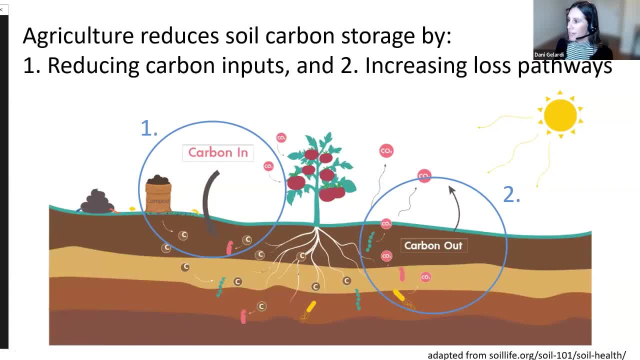 So let's go over both of these kind of important facets of agriculture. Let's talk about first the inputs. Plant breeding techniques are actually a really big driver of reduced carbon inputs. Over the years, breeders have developed crops that are optimized for maximum yield, And this is great, again, because we have to feed a growing population. 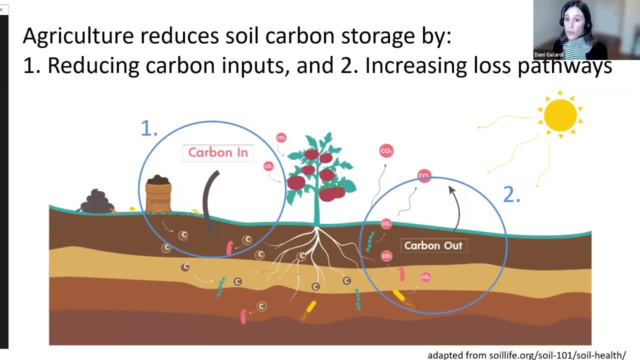 However, it does mean that modern varieties often promote the growth of grain or fruits which are harvested out of the field, rather than growing out of the field. So we have to keep in mind that we're not only going to be producing crops that are harvested out of the field. 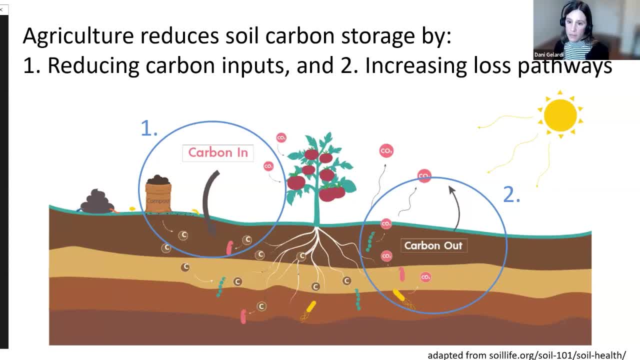 but we're also going to be using crops that are coming from the field. So we're going to be using crops that are coming from the field, but we're also going to be using crops that are coming that aren't harvested like stover or stock. So crop management also contributes to this issue. 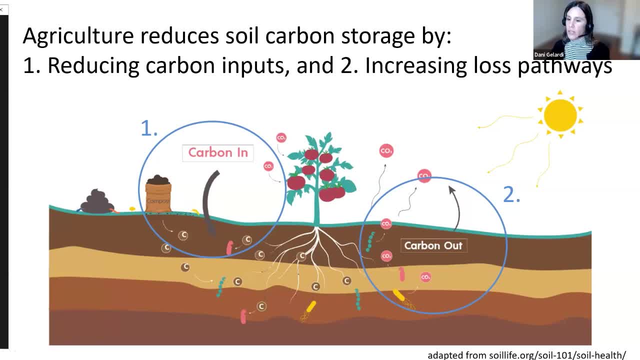 For example, removing crop residues like corn stover and wheat stalks rather than returning them to the field. In eastern Washington, for example, someone may harvest their wheat and then secondarily come through and harvest their stalks to sell them to a paper pulping facility, And this 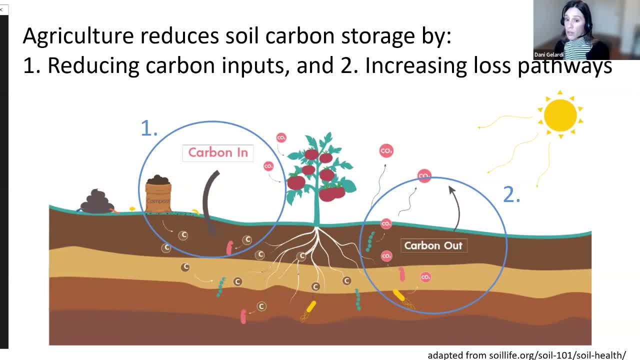 is great secondary income, but it also removes a lot of carbon from the field and other essential plant nutrients And, of course, agriculture increases loss pathways. I think this is the piece that gets talked about more in kind of the popular press. Mechanical tillage exposes carbon. that was once. 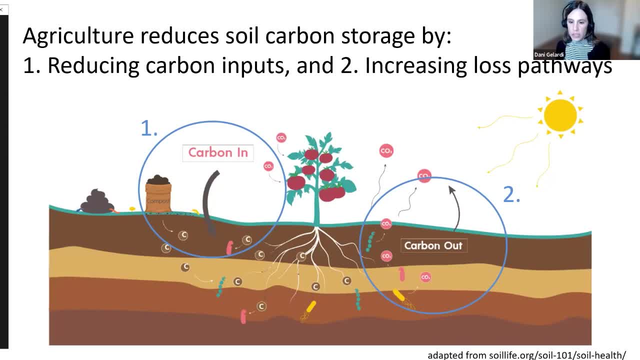 protected to oxidation and mineralization and erosion. The burning of crop residues can destroy soil organic matter at the soil surface. Even things that are necessary, like irrigation, can result in soluble carbon leaching through the soil and into the groundwater or nearby surface waters. Soil not held in place by ground cover or living roots, such as in fallowed fields. 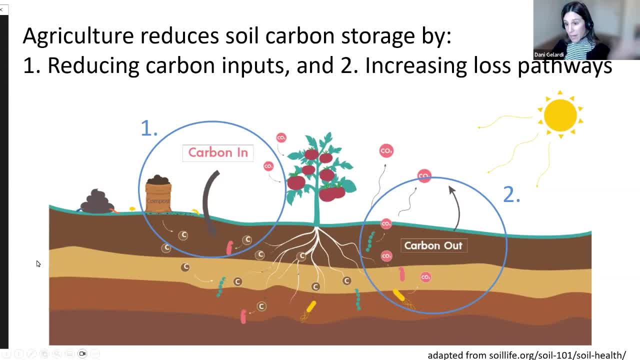 can be lost through runoff and erosion, which can carry carbon with it. And you know, unsurprisingly, when you look at these two together, this can lead to an overall reduction in our carbon stocks: Reduced carbon inputs, while increased carbon outputs leads to reduced storage. 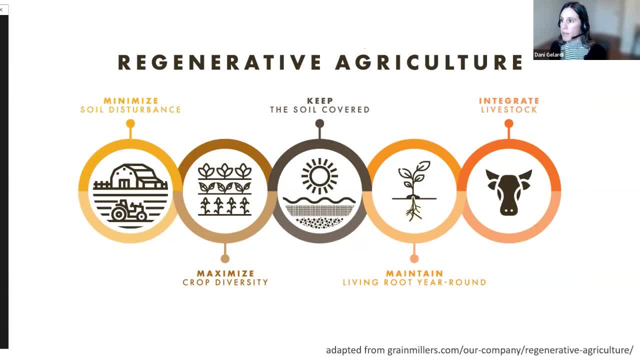 But there's hope. A lot of people here have been working in the regenerative agriculture space- things like carbon farming or climate smart agriculture. regenerative management: These terms help define a suite of practices that are aimed at optimizing crop production while protecting and building soil organic matter. 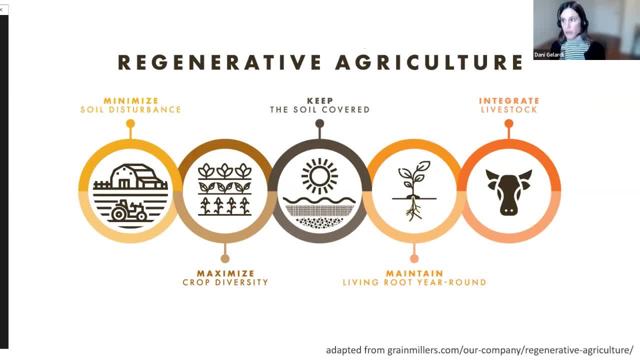 These practices tend to relate back to the five soil health principles: Minimizing disturbance, maximizing diversity, keeping the soil covered, maintaining a living root year-round and integrating livestock. So those are the kind of big principles, but actual practices include things. 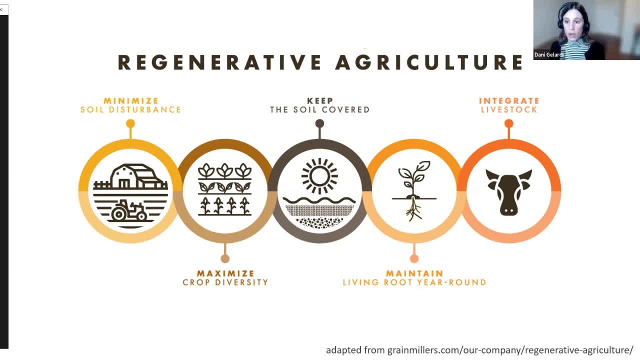 like reducing tillage, reducing fallowing cover, cropping adding carbon-based fertility like manure, compost, crop residues, biochar and even more out-of-the-bottom practices like seed boxings, like trying to breed crop varieties that produce more roots and root exudates. 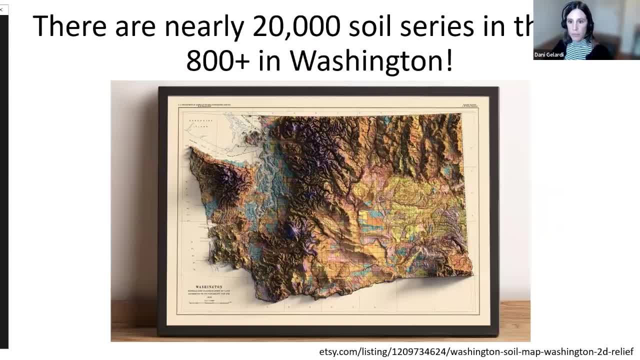 or retiring marginal lands from production. While these practices are incredibly important for promoting soil health and providing ecosystem services, it's important to remember that they are not a one-size-fits-all solution for increasing soil carbon storage. Soils are incredibly diverse: There are nearly 20,000. 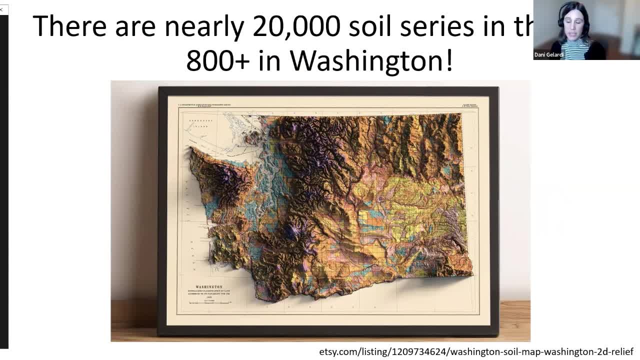 soil series in the United States with over 800 here in Washington, And that means that even within a single field there will be great variation in the potential for management to increase soil. carbon Management is an important variable, but there are a lot of. 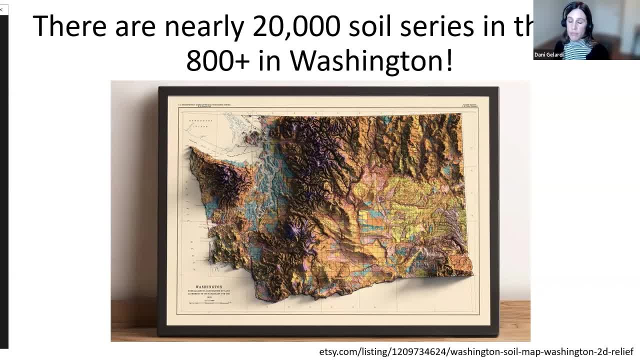 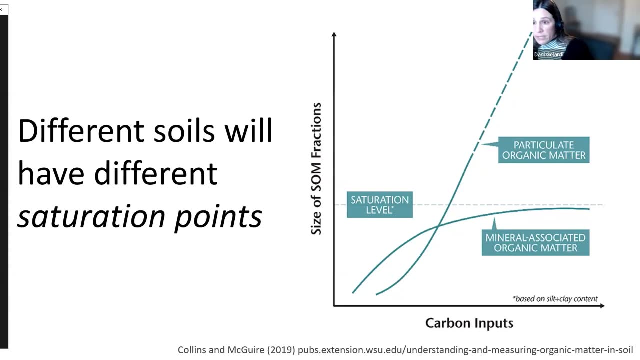 variables that are beyond our control, Things like soil texture, mineralogy and climate, things like precipitation and temperature, that cannot be changed through regenerative agriculture practices, For example. potential increases in soil carbon are not infinite. Many soils will have a sort of natural equilibrium, what is frequently called 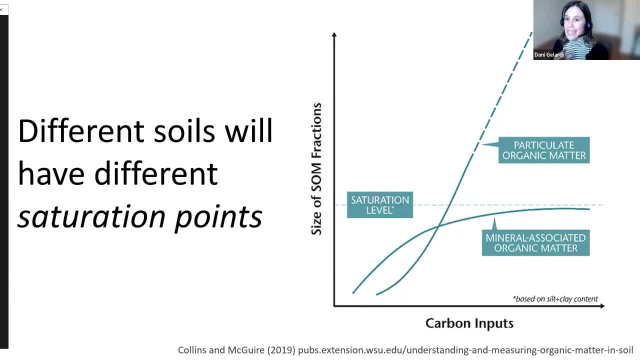 a saturation point after which the gains as a result of management can plateau or sort of level out, And this will be different in different soils: Soils with more clay or more reactive clay minerals will have higher carbon carrying capacity, And, of course, soils that are already. 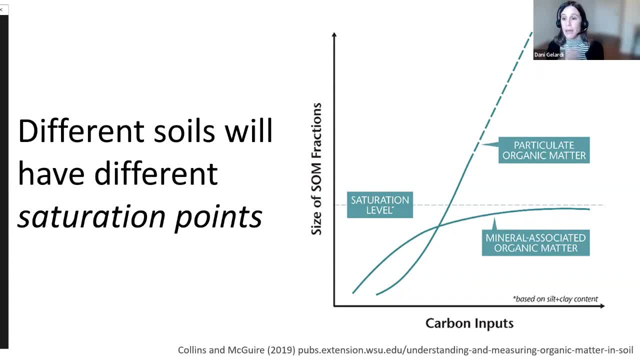 degraded or very low in soil carbon will be able to gain carbon quickly, And so perhaps the soil that's already at or near its saturation level, Much of the carbon that's added after this is still important, because it helps feed microbes in this kind of particulate organic 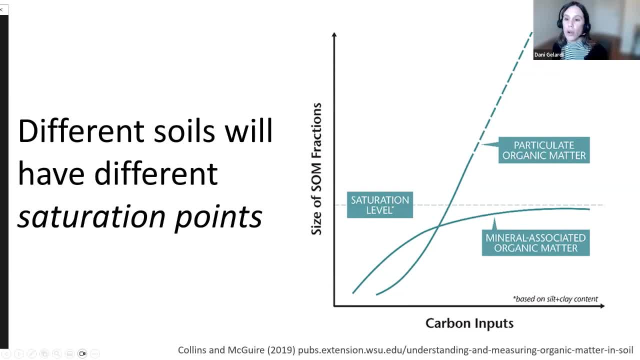 matter phase. However, it's a lot harder for that carbon to be stored in a more recalcitrant form to increase overall soil carbon stocks. You may also remember your stoichiometry lessons from high school And I'm sure you've learned a lot from that. So if you're interested in 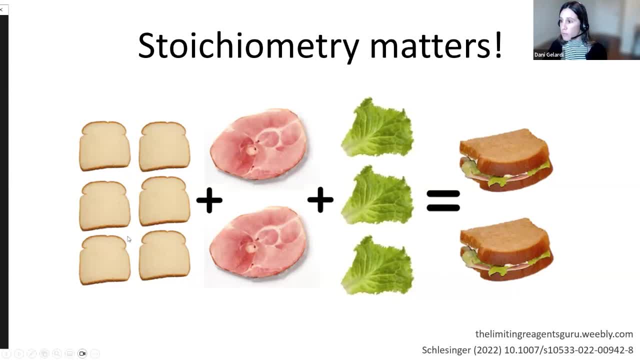 this kind of math, go to our website at brainatedu And you can get all the information in a few minutes. So if you're interested in this kind of math, go to our website at brainatedu And you can get all the information in this kind of math. So if you're interested in, 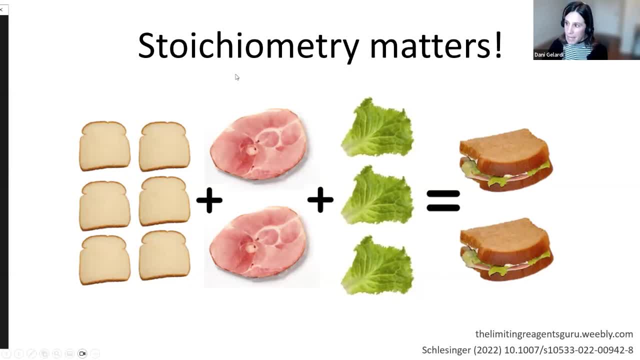 this kind of math, go to our website at brainatedu And you can get all the information in here. we have only enough ham. I think that is to make two sandwiches, And so we only get two sandwiches. And it's no different with soil, carbon storage, Other essential nutrients like nitrogen. 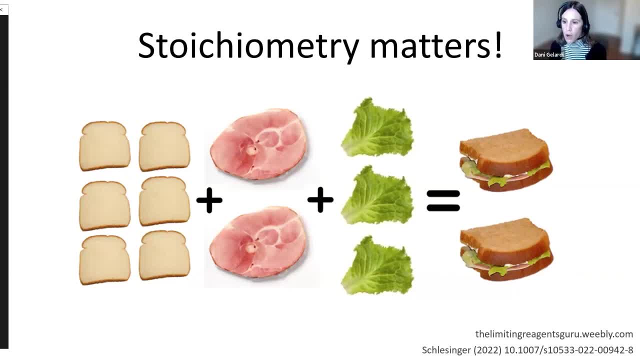 phosphorus and sulfur are required for the conversion of carbon inputs into soil organic matter. Remember that soil organic matter is only about 58% carbon, And so we need to those other ingredients as well. That means that in some cases, practices that literally add carbon. 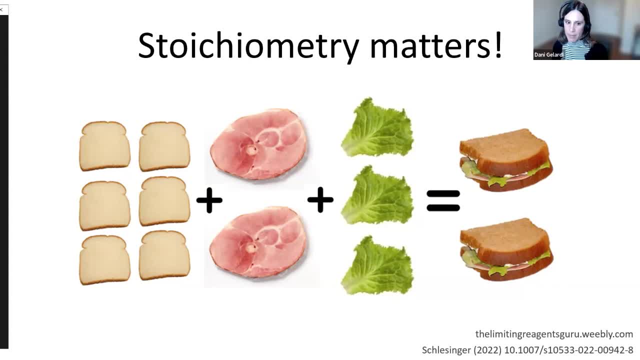 to the soil do not necessarily build soil organic matter or achieve increased soil carbon storage if other inputs are not also present. I've included a link here, this bottom paper, to a paper, a recent review paper, that really highlights how essential stoichiometry is for building soil carbon. 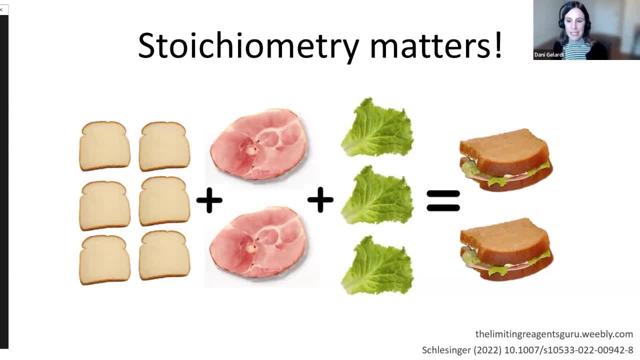 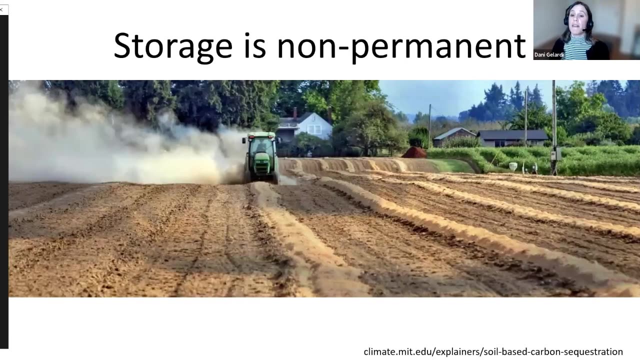 and sort of goes through the different regenerative agricultural practices with a stoichiometry lens, And throughout this presentation I've included some papers that are relevant. I'm also happy to share resources if anyone wants to talk about them later. The final complicating factor I want to point out is that soil carbon storage is not permanent. 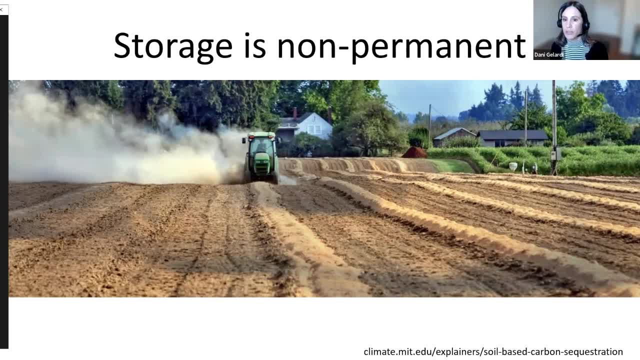 Remember it is a cycle. Even that stable, recalcitrant mineral, associated organic matter can be lost. This means that you could spend a lifetime trying to accrue soil carbon only to have it lost in a few years through intensive management or other unforeseeable events like a well going dry or several drought years. 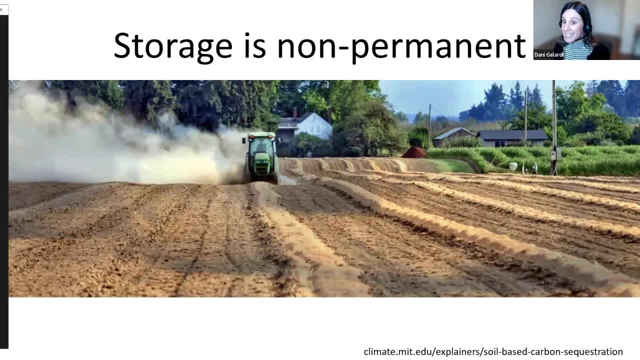 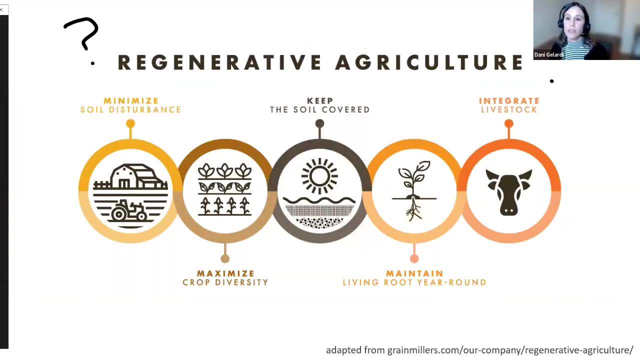 or heat domes, And this really highlights the importance of sustained land tenure and having policies and programs in place to incentivize long-term stewardship, because an increase in one year is really, really important but can be reversed in the next year. So let's go back to our regenerative agricultural principles and practices. 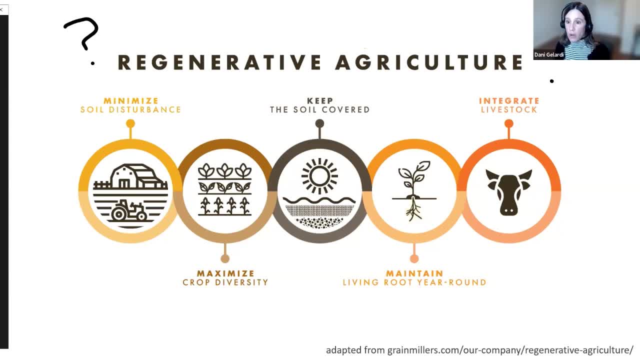 It's not surprising that they don't all increase soil carbon in all conditions. I can't go through individual studies, but again, I'm always happy to share resources. But briefly, there have been studies that show, for example, conservation tillage has increased, decreased. 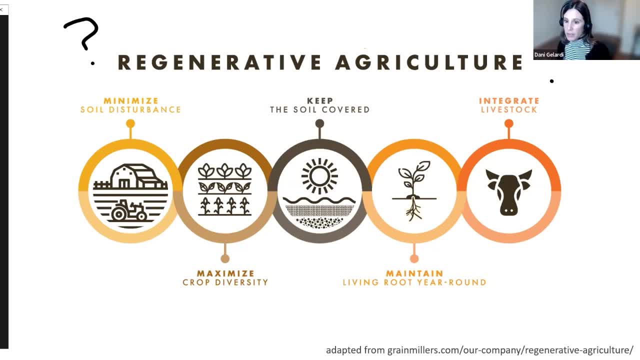 and had no effect on soil carbon, depending on a lot of variables. In fact, one meta analysis determined that reduced tillage across all conditions evaluated globally, actually reduced yields by an average of 5.1%. And, of course, reduced crop yields may require more land be converted to agricultural production. 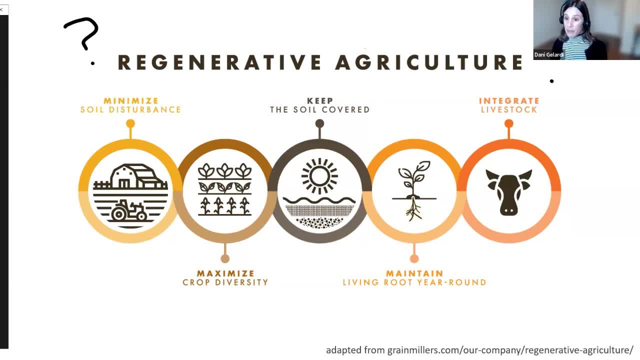 That may mean deforestation or native prairies being put into production, which of course results in a net soil carbon loss overall. Another example is that the impact of cover cropping on soil carbon has been observed to be pretty specific to the conditions. So fine texture soils have a greater impact from cover cropping. 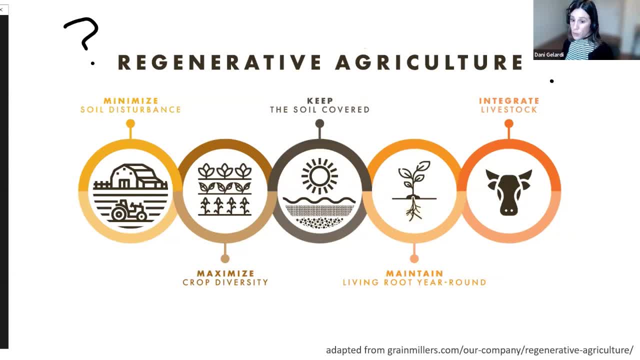 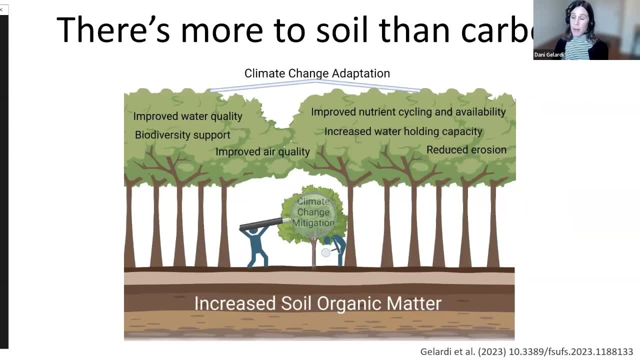 And because of stoichiometry when a nitrogen-fixing legume is also present in the cover crop species mix. This is why I like to talk about soil health and not just soil carbon, because conservation practices deliver benefits beyond just soil carbon sequestration. I encourage people to not miss. 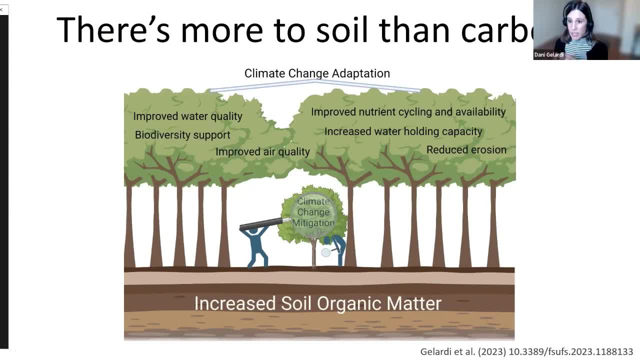 the forest for the trees. I encourage people to not miss the trees and think only about climate change mitigation, but in fact, climate change adaptation and the role that these practices can play in helping producers and society stay resilient through a climate changing climate and helping us adapt. 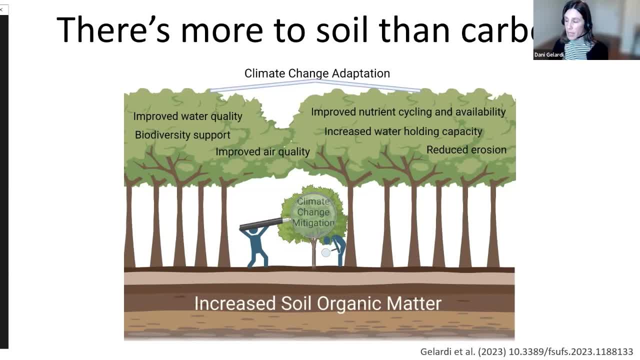 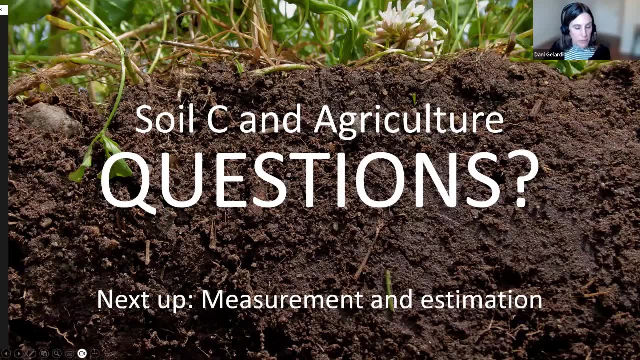 to climate change, even in cases where these practices don't mitigate climate change. All right. next up, we are going to talk about measurements and estimation, and I see a few questions in the chat. So what role does water holding capacity play in soil? carbon sequestration? That's a great question. 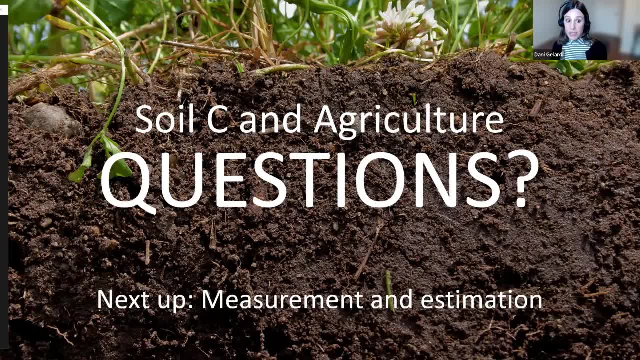 and one that really highlights how important these kind of fixed variables are. It is a lot easier to build soil organic matter when you have irrigation or when you can sort of stimulate soil microbes and decomposition through a solid water supply. So what role does water holding capacity play in soil? 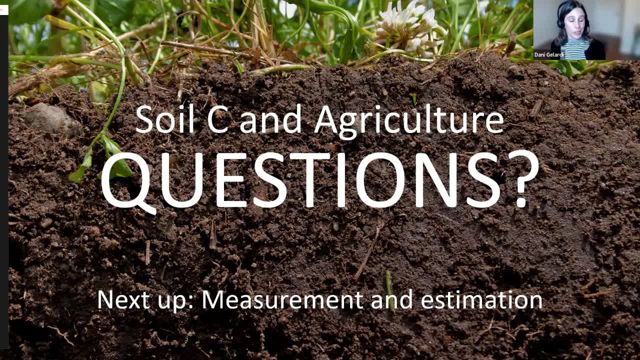 carbon sequestration. So what role does water holding capacity play in soil carbon sequestration? That's a great question. So it's a bit of a feedback loop where more water can help you build soil organic carbon and soil organic carbon can help you store more water. So it's a lot harder in a dryland context and this is 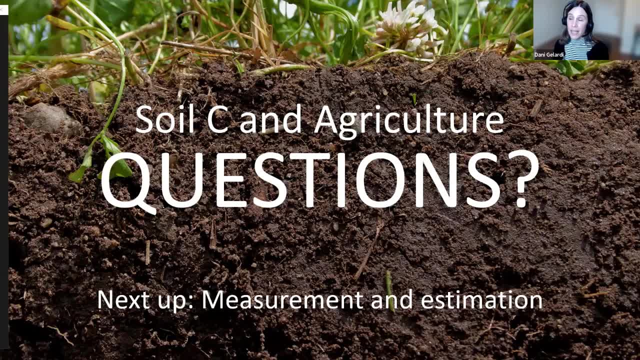 very easy to see in Washington, where on the east side, where there's a lot of dryland agriculture, you may have soils that are just below one percent soil organic matter, whereas on the west side, where water is not typically limited, 8 percent soil organic matter. 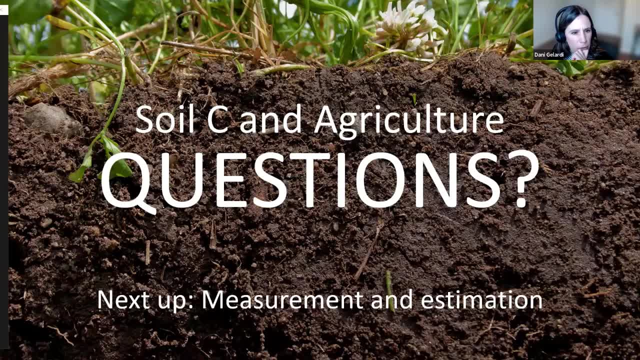 And I have another question about CO2 fixing microbes. I'm not sure I totally understand the question, So at the end, Victor, I encourage you to ask it. I think we may cover some of this in the next section, but I also am happy to talk more about it. 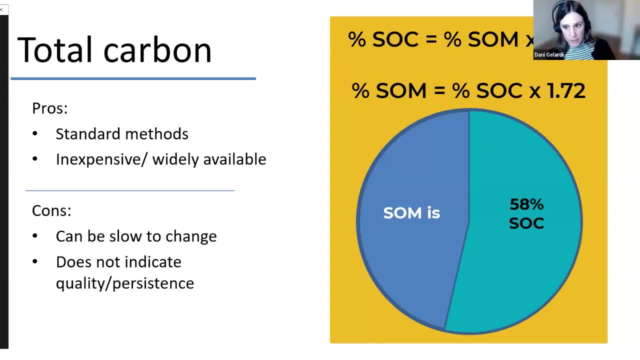 Okay, so now we're going to talk about measurements. I've mentioned many times that soil carbon is contained in what we tend to call different pools that are stored in the soil for variable lengths of time, And so let's talk about some of the ways we measure those pools. 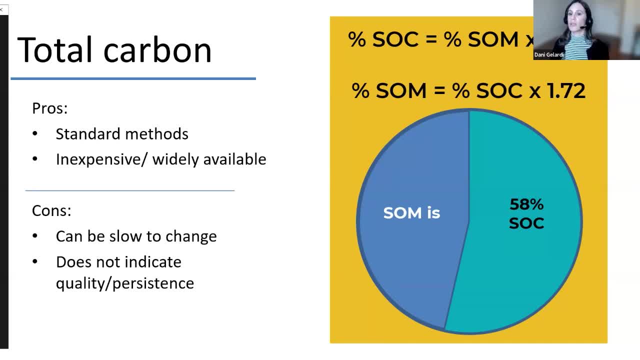 The most commonly tested carbon pool is called soil organic carbon or SOC. Again, that's about 58 percent of soil organic matter, SOM. If you do not have carbonates in your soil, you may also get a result back that says this is: 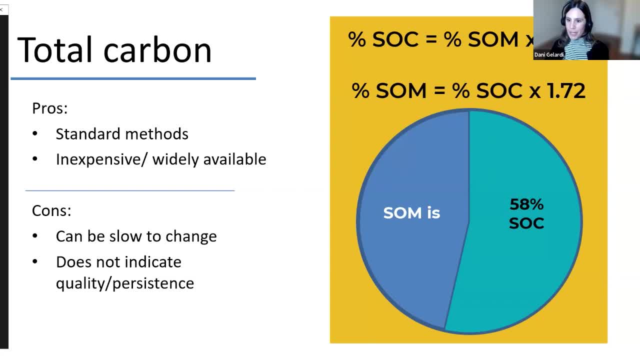 total carbon or TC. It's a lot of acronyms to remember, But fortunately you do not need to measure all of these If your lab has only SOM or SOC, that's okay, because they're really easy to convert back and 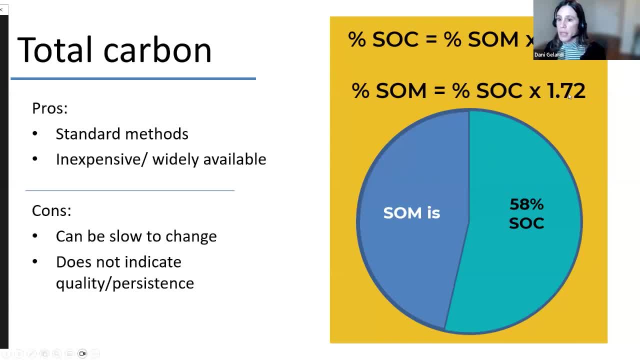 forth using these calculations. So the pros of this is that it's a very old method. It's a very common method for different kinds of contamination. Our lab doesn't let you measure, accomplish those old method. It's pretty standard. You can get it at any lab, pretty much anywhere. It's not so. 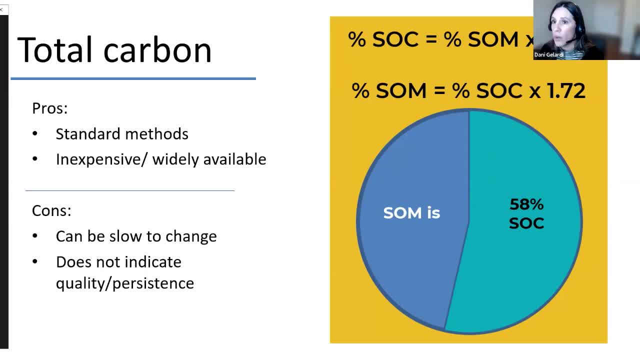 expensive and you can pretty reliably know that your lab has honed in on the same SOP or standard operating procedure, as any other lab you send it to. The cons of this measurement, however, are that it can be slow to change, So if you have implemented a new practice in your fields, 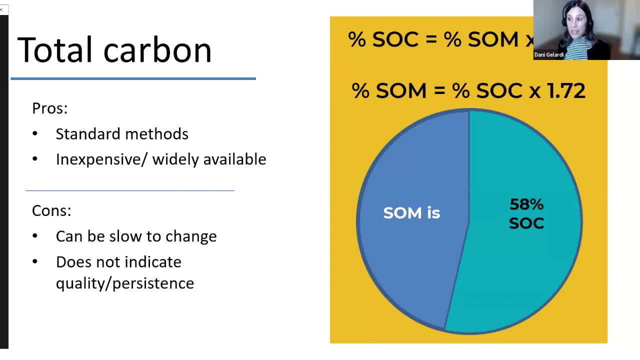 and you want to see the impact of carbon after one year. soil organic matter may not be the best measurement because it takes kind of a long time to build soil organic matter. The other con is that this measurement does not help you know anything about the quality of that carbon or the persistence? 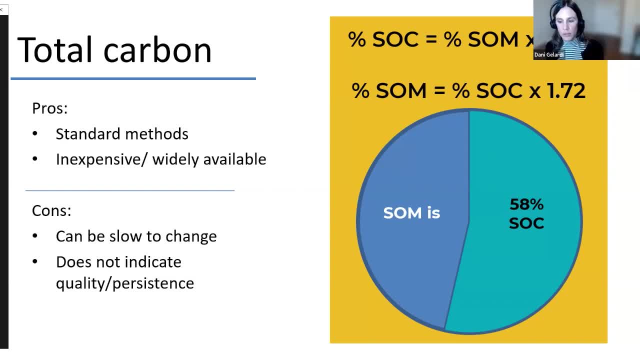 For example, you could get a result that shows you have really high soil organic carbon when you accidentally just took a soil sample that had perhaps an animal just defecated there, or perhaps you just added compost, and so you're really measuring compost carbon, which will quickly decompose. Honestly, total carbon can even pick up on. 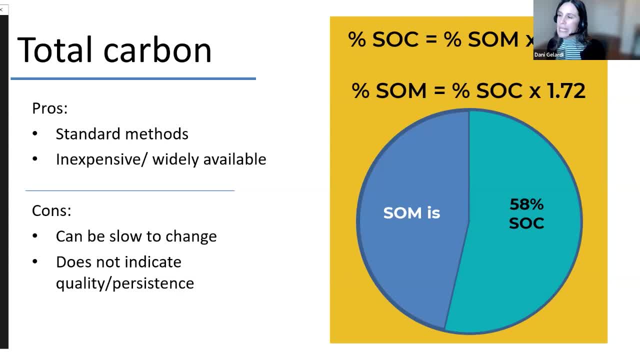 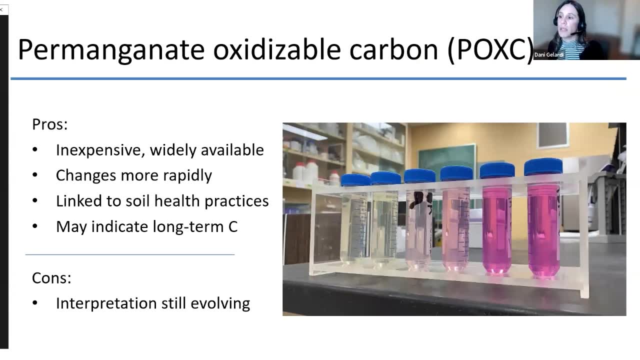 things like microplastics, which are carbon-based, and so this doesn't really tell you a lot about the persistence of your carbon. However, there's a lot of new measurements coming online that help you get more at that quality or persistence. Permanganate- oxidizable carbon. 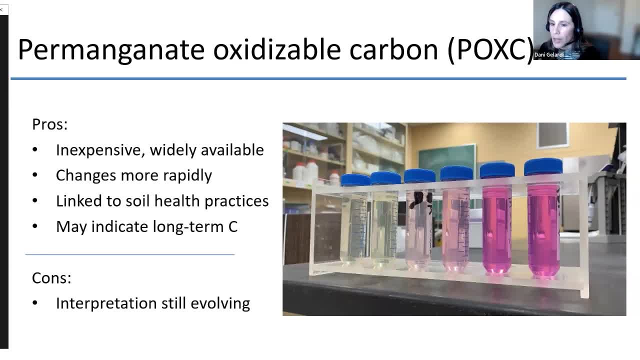 often called POXI, measures the amount of carbon that is oxidized by a very strong oxidizer called permanganate. This is a newer test aimed at learning more about soil carbon quality and persistence. This measurement was once called active carbon because for a while. 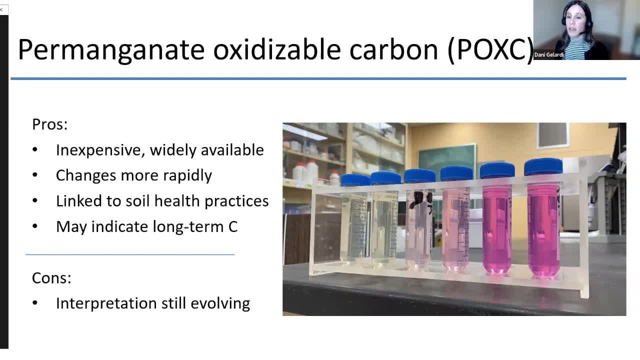 it was believed to represent the fraction of carbon that was available for microbial consumption, But in fact the opposite interpretation has emerged in recent years. Comprehensive studies just this year actually have showed that POXI is actually measuring much more stable forms of carbon, Things like phenolic and aromatic compounds in lignin, for example. So these compounds are not. 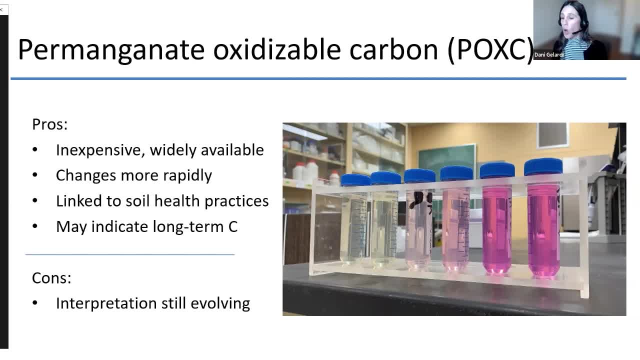 necessarily microbially available, but actually likely already processed by microbes. This is actually really exciting, because what it may indicate is carbon that's on its way to becoming stored for the long term. This method also changes more rapidly than soil organic matter, So perhaps if you after only one or two seasons, 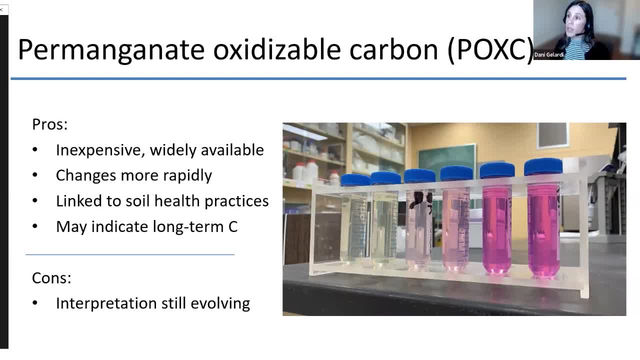 of a management change, are curious about what it's doing to carbon. you want to look to POXI instead of soil organic matter, And it has been linked to soil health practices, with more conservation practices having more POXI, So it's an exciting new measurement. However, 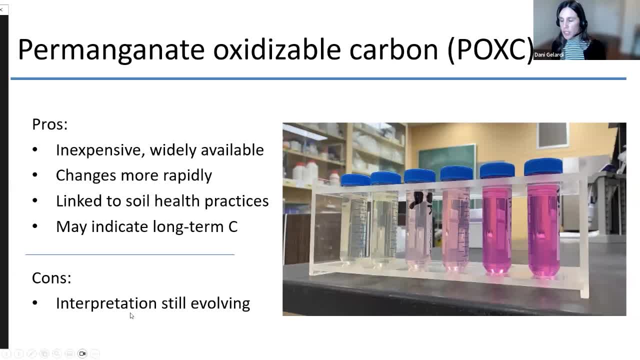 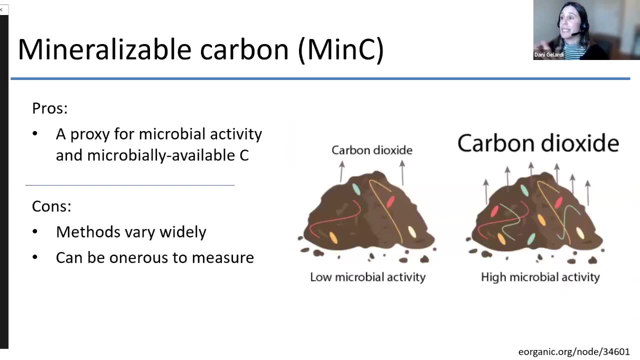 the con is that it is new and our interpretation of it is still evolving. If you got a POXI measurement five years ago, what they told you it meant would be different than what they tell you it means today, And so we're kind of all on this journey together. Mineralizable carbon is another. 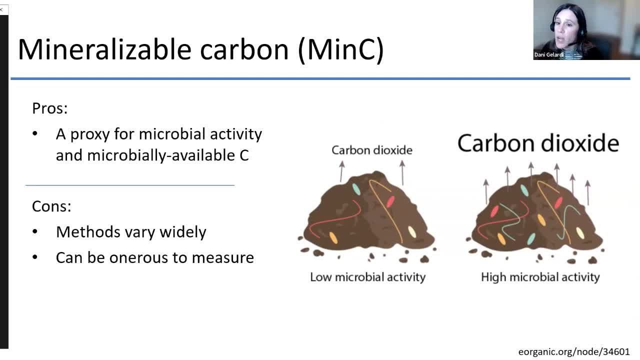 popular measurement. This is the carbon dioxide given off of soil after rewetting in a soil incubation. It's often called respiration or solvita burst test. This is an exciting measurement because again, it sort of centers microbes, soil microbes and 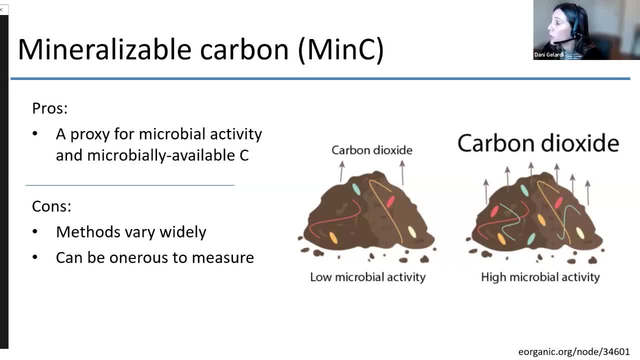 how active they are and how much available carbon they have. The cons to this method again are that it's slightly newer and the methods vary really widely Depending on what lab you measure it at. they may use a one-day incubation or a four-day incubation or anywhere in between. They 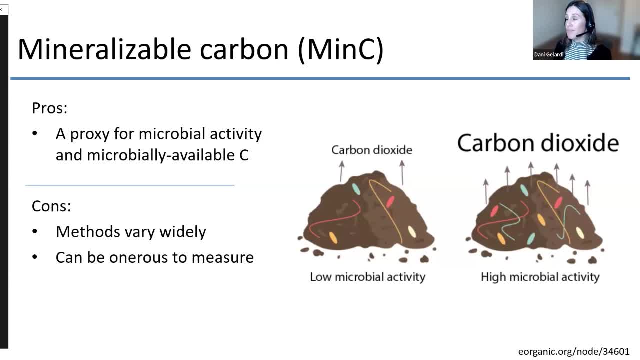 may also keep it at different temperatures or incubate it at different water contents. So you really want to make sure to be using the same lab consistently if this is the measurement you're interested in And it's not available at all labs, because it can be onerous to measure Babying little. 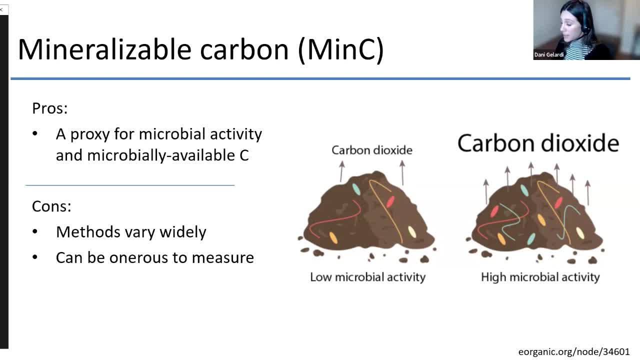 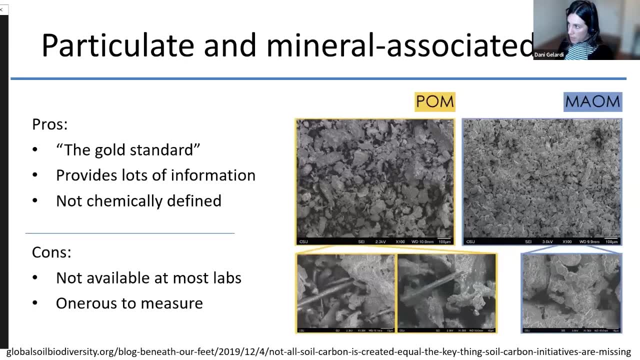 soil. incubations for four days is not necessarily everyone's idea of a good time, So you won't see this at all. labs, Particulate and mineral-associated organic matter are another measurements that are important in this discussion. You've heard me talk about MAOM and POM And this. 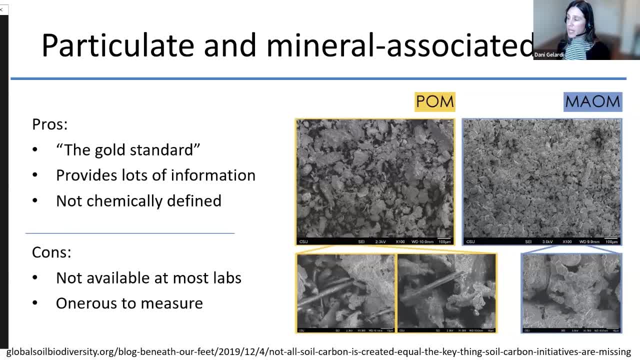 is really considered the gold standard of carbon measurements. It provides a lot of information. This measurement tells you what of your carbon is associated with minerals, and so how much of it is likely very stable and how much of it can be lost through microbial processing and 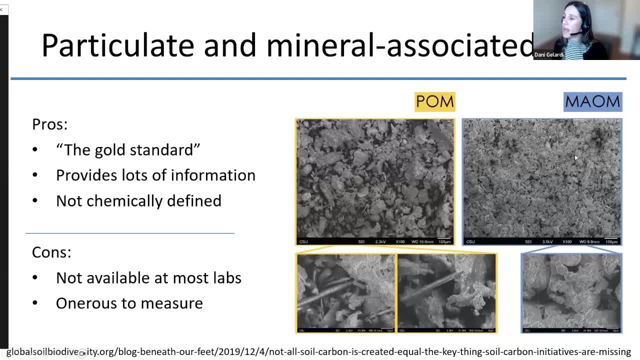 mineralization- or hopefully can make it over into the MAOM category- Provides a lot of information. It's also not chemically defined, So remember those humic substances we talked about. This doesn't expose soils to harsh chemical extractions and, in fact, is really just a size. 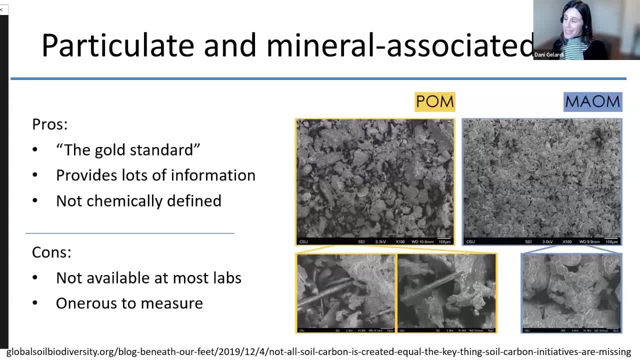 fractionation. The cons of this method are that it's not really available at almost any labs. You really have to be working with a university researcher to get these measurements, at least at this stage, because it can be onerous to measure. 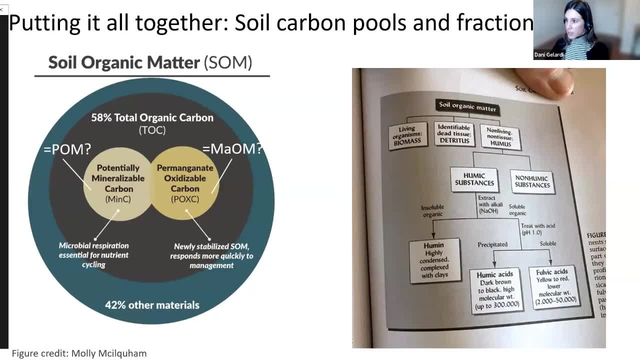 So we're going to put all of those pools together in a single figure: Soil organic matter, this big blue circle, 58 percent of which is soil organic carbon. Within that we have different pools: potentially mineralizable carbon and permanganate oxidizable carbon. Those are not necessarily distinct and 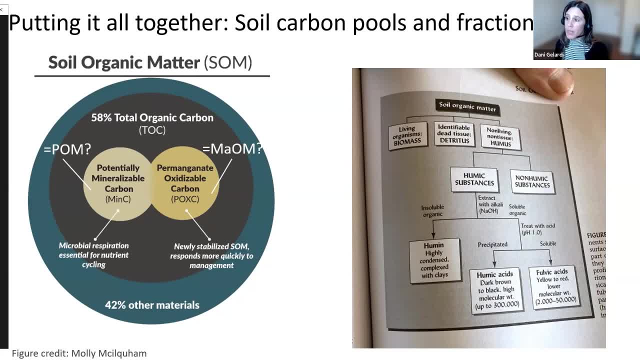 may have overlapping components to them. There's also POM and MAOM which at this stage, may be well correlated with MNC and POXY. There's a lot of research to indicate that POM is measuring MNC And MAOM is measuring POXY or- sorry, vice versa- POXY is measuring MAOM, MNC is measuring POM. 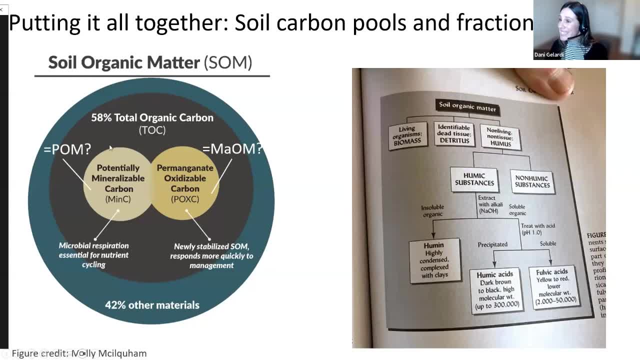 All of that means is that, even though you may not be able to measure these things in your lab- POM and MAOM- it's possible that POXY and MNC, which are more available, are sort of getting at that, And that's an evolving area of research. If that sounds like a lot, it is. It definitely keeps. 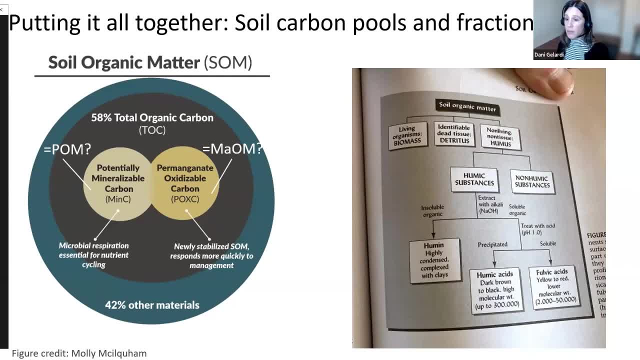 me up at night. These measurements are at the cutting edge of carbon estimation and measurement, but we have to remember that we're not going to be able to measure all of these things at the same time. We have to remember that our understanding and our scientific capacity is changing all the time. 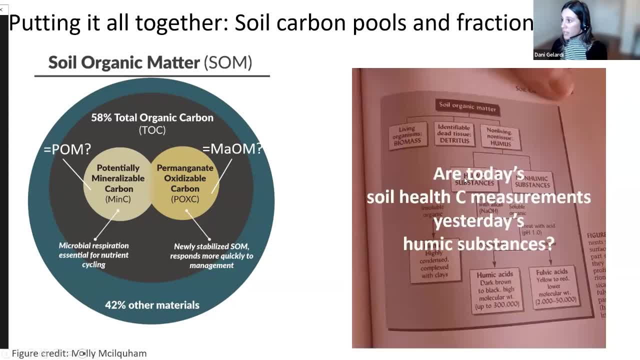 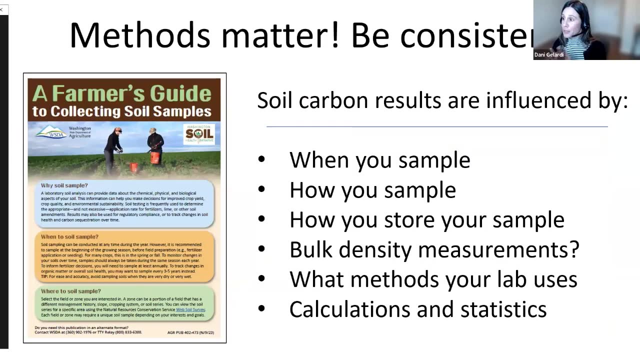 Recall the humic substances of yesteryear. It's quite possible that one day in the future, today's soil health carbon measurements are similarly considered obsolete. So again, we are sort of all on this journey together, But there are a lot of things that you can control. 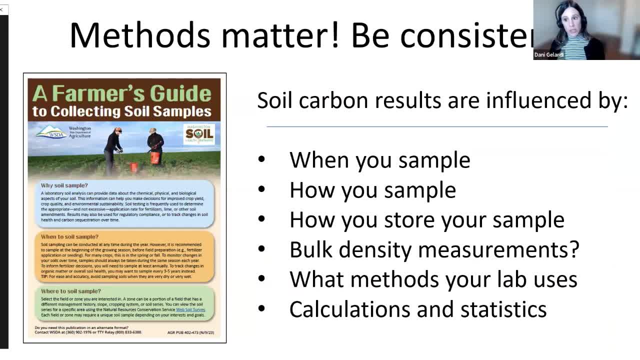 So I want to talk about sampling methods. There are more decisions to make than just which measurements to take, So I want to talk about sampling methods. So I want to talk about sampling methods. So methods matter, And let's talk about those different methods. Your soil carbon results are. 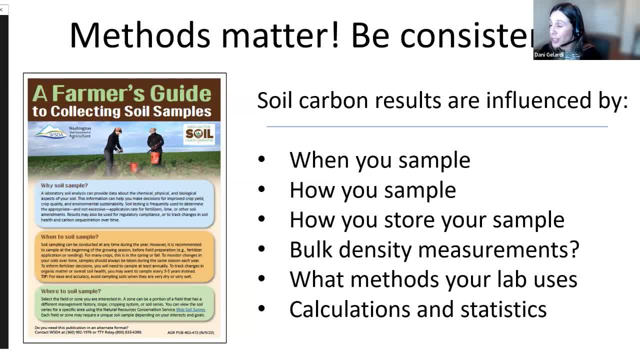 highly influenced by when you sample. There's research that shows that soil carbon measurements have a sort of seasonal flux- up to 14% in some conditions, And so if you sample in the spring in 2023, you want to make sure you sample in the spring in 2024, so that the difference you see. 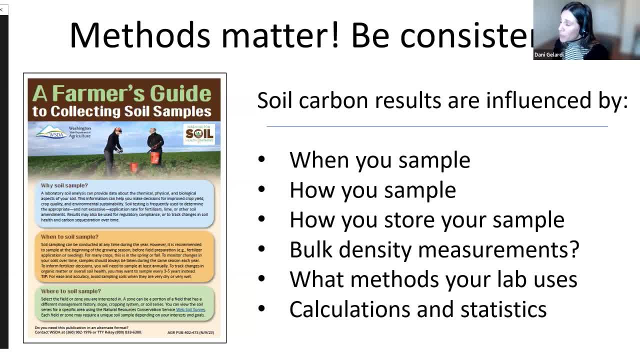 isn't just about the amount of soil you sample. You want to make sure you sample in the spring in 2023,. you want to make sure you sample in the spring in 24 years. How you sample matters. how you store your sample matters, If what you're interested in is microbial mineralization. 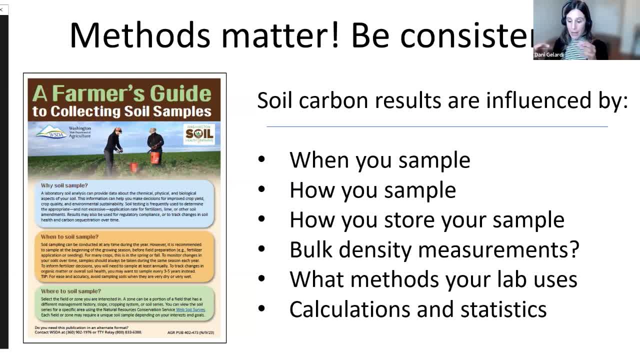 you don't want to seal your sample in a bag where you're creating anoxic conditions and basically lysing all of your microbes. If you are interested in soil carbon stocks, so not just the percent of carbon but the actual quantity in your soil overall- you have to measure. 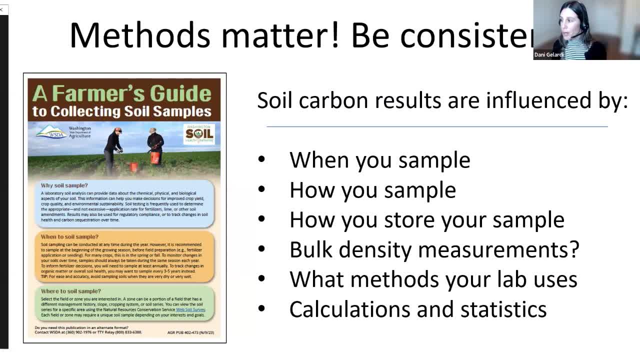 density, And that is not an easy thing to measure. There are a lot of methods, a lot of challenges- That's for a whole another webinar, But note that that is one of the variables- And, of course, what methods your lab uses and the calculations and statistics you use to calculate things like 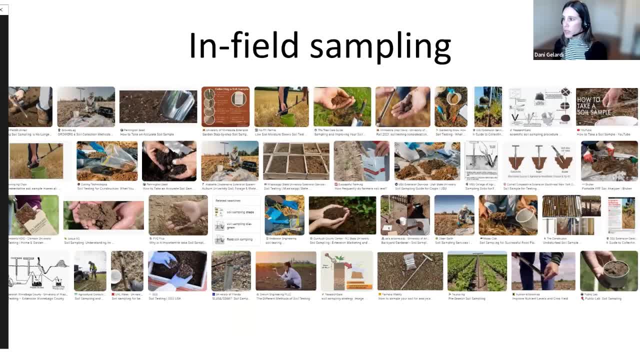 soil, carbon stocks. Infield sampling, of course, is the most common. If you Google it, there is a million different resources about how to do it, when to do it. The pros of this are that you are actually taking your soil and sending it to a lab and getting a measurement for your soil. 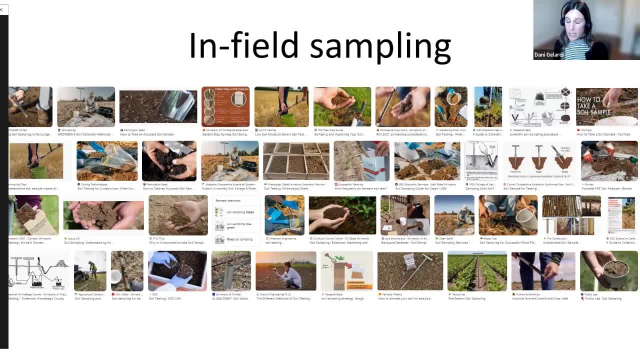 The cons, of course, is that there are a lot of decisions to make. Recall that soils store carbon differently based on texture, depth, mineralogy, climate, even within a single field. So taking sufficient samples to account for variability can be prohibitively labor and cost intensive. 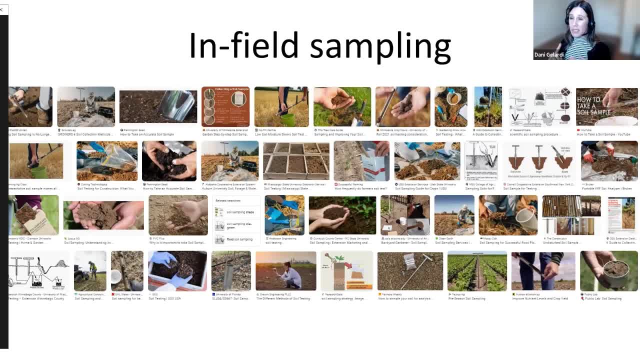 You have to decide how many samples do you take? How many subsamples goes into each sample. You have to decide how many subsamples goes into each sample. You have to decide how many subsamples goes into each sample. You have to decide how many subsamples goes into each sample. 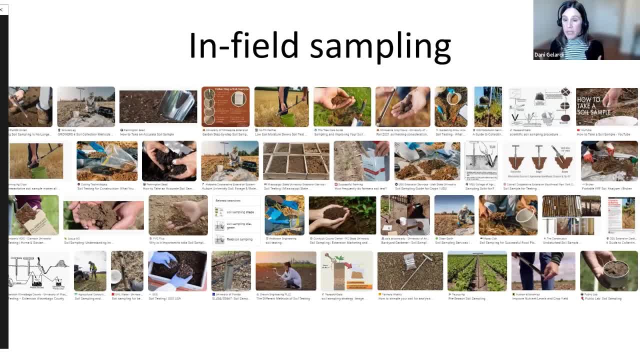 And, importantly, how deep will you sample? It's common to sample only from the soil surface, but there is so much carbon that exists all the way down to the bedrock, And so you know if you're sampling only the top 6 or 12 inches, this can lead to false conclusions- that carbon 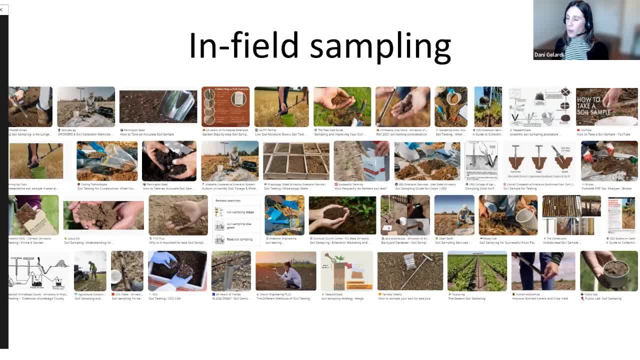 is being lost or gained as a result of management, when it's actually just being vertically redistributed. So we'd like to sample all the way to bedrock every time we take a sample, but of course 6 or 12 inches is just what's more practical. 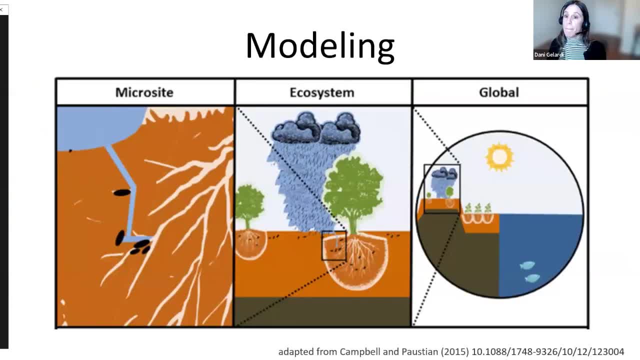 Luckily, there are other strategies. Soil carbon modeling may be a strategy to kind of overcome all of the challenges of resource intensive soil sampling. You are probably familiar with models like CropSys or Comet Farm which can estimate the carbon sequestration potential without soil sampling. However, for models to be built at all, they do have to incorporate 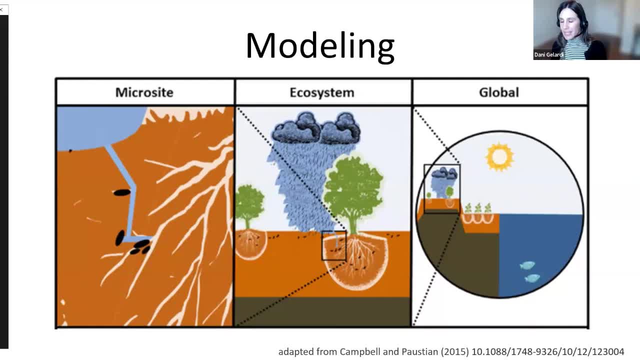 existing sample-based data sets, So their accuracy hinges upon data quality and availability in any given region, And there are many, many variables included in the models. Does your model include factors like crop type? Comet Farm does, but Comet Planner does not? Does your model include? 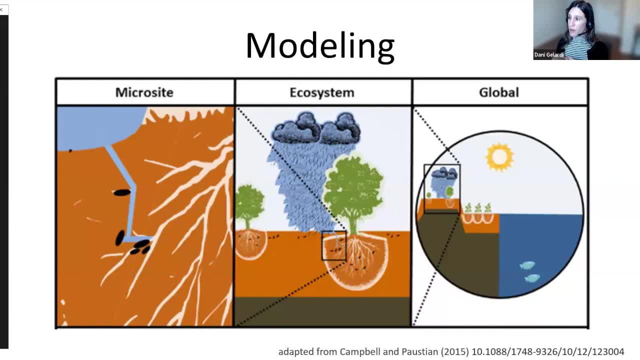 the influence of microbes or mineralogy, whether or not plant litter is returned to the field. What depth are you modeling And does it model the fact that we are in a changing climate and things are getting hotter and drier? Not all models include all of these factors. Also, can the user input site-specific. 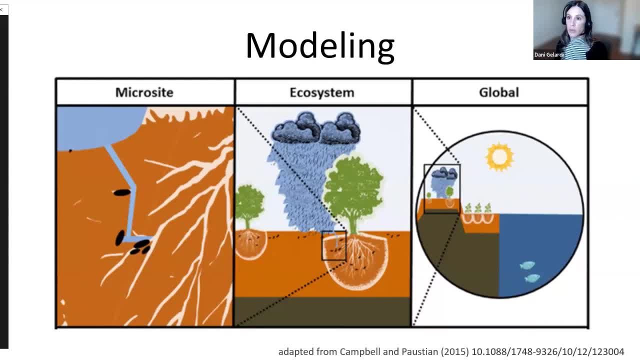 data? For example, if you already know you have 2% soil organic matter, can you start your model by entering that number or does it just assume based on publicly available data sets? Models are great because they provide swift and inexpensive estimates and they spare. 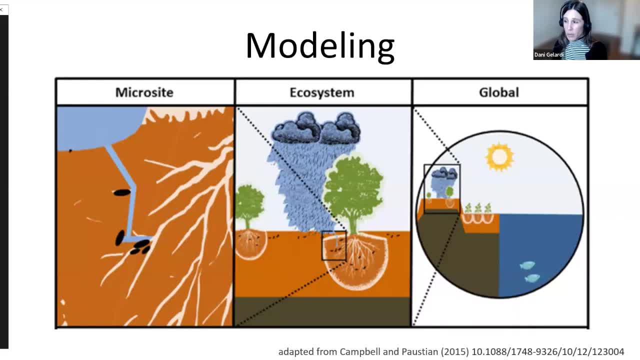 technical assistance providers from having to go out and soil sample, So overall they reduce monitoring and verification costs. However, they have variable success in making accurate predictions due to all of the different variables we've talked about, And over-reliance on models can. 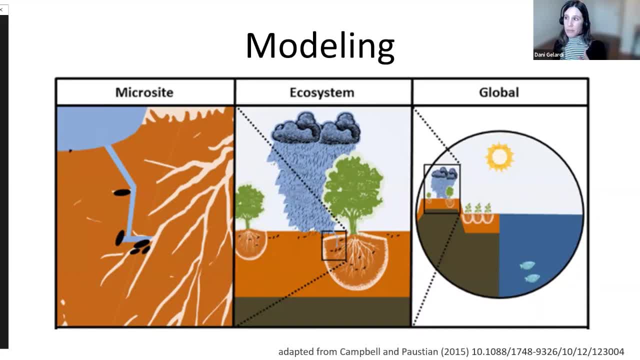 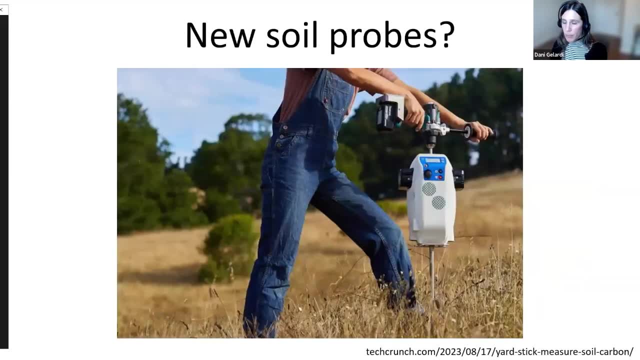 contribute to inaccurate estimates and some bigger social challenges, which we'll talk a little bit about when we talk about soil carbon markets. next, There's new technology coming online. So, for example, there's a company called Yardstick- this is their probe here- who have built a probe that can measure soil carbon down to. 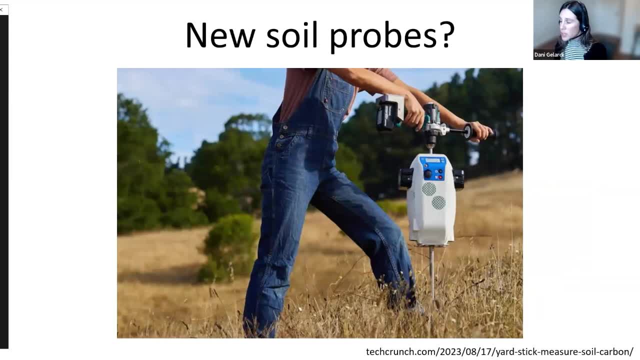 three feet using infrared spectroscopy. There's other spectroscopy methods too, where there's like a little roving robot that you can put a sample in and in the field it can measure. This is great because instead of collecting sample after sample and then sending it to, 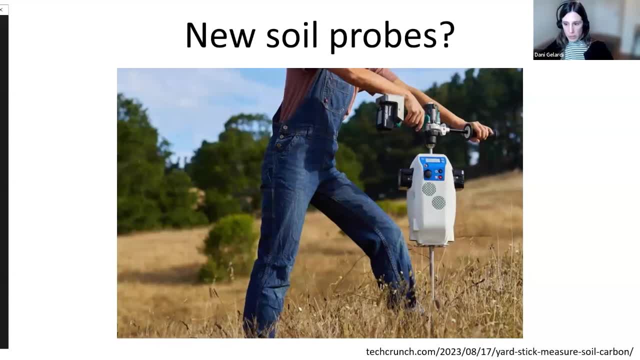 the lab and waiting for results, you can just stick the probe in the soil as many times as you'd like and account for all of that variability. And in fact spectroscopy has been deemed reliable enough to be added as an acceptable quantification method in new VERA soil carbon protocols. 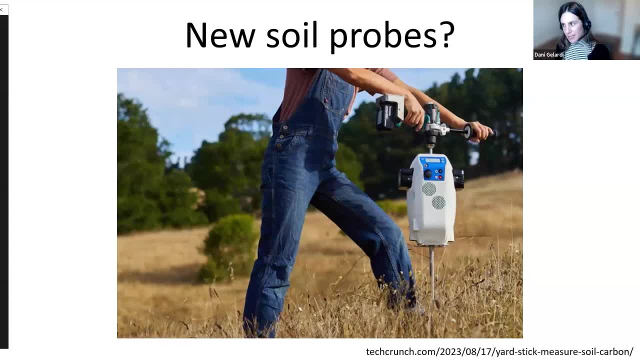 But of course this is new technology, so you're not likely to see one of these at your conservation district, at least not today. The technology is nascent, it's not yet widely available and I have no clue on what something like this may cost. Many of you are. 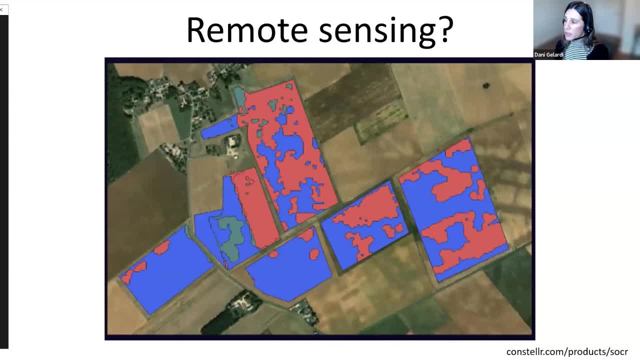 familiar with the use of remote sensing in agriculture, particularly through NDVI measurements, which uses spectral wavelengths in the near-infrared and visible ranges to estimate different aspects of plant health, And researchers at universities and in the private sector are attempting to use the same technology on bare ground to estimate soil carbon. This is still 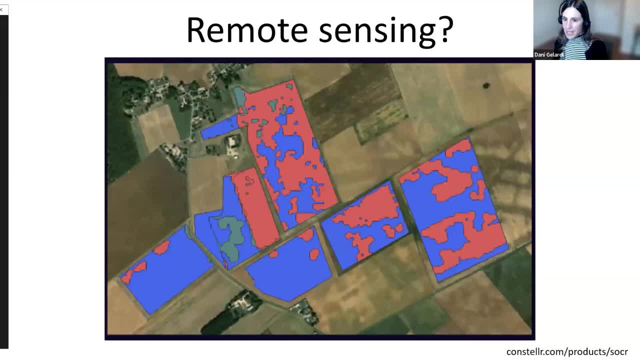 a fairly new field, but it has a lot of potential. Imagine being able to use existing satellite imagery to estimate soil carbon. This is a new field, but it has a lot of potential. Imagine being able to use existing satellite imagery to estimate soil carbon. 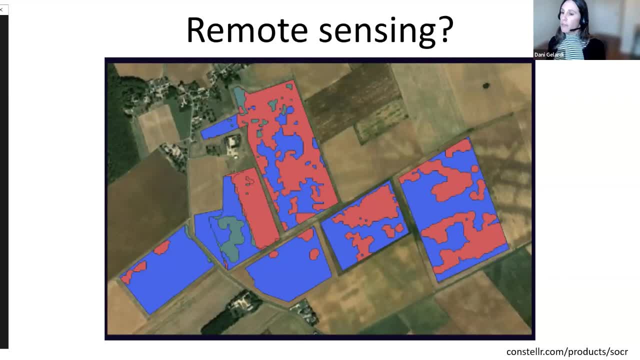 stocks and not needing to take samples at all. Of course this is developing and there are a lot of unknowns. For example, how deep can satellite images really detect soil carbon? How much does soil moisture impact? what signals the satellites are getting? You know there's a lot that folks are still. 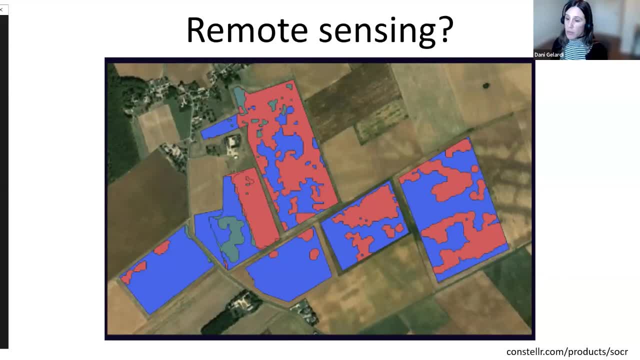 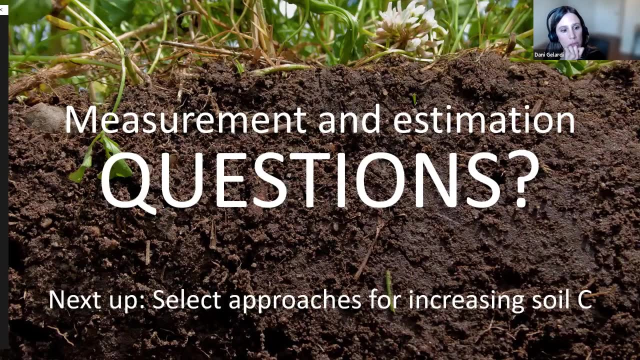 researching And in fact, there's a team at Washington State University working on this very issue as we speak. So looks like we do not have any new questions in the chat. I do hope to have some time at the end for discussion, So we are going to go into our final question, which is: how do we increase soil? 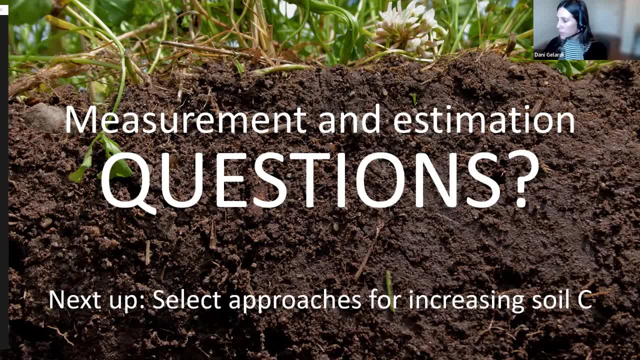 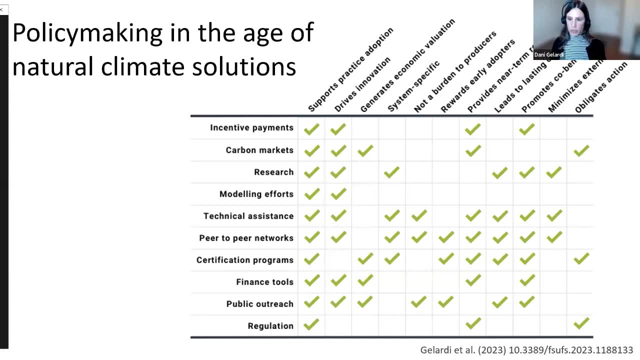 carbon. So you can imagine that, with all of the complications in building and measuring soil carbon Making policies and programs to promote soil carbon storage is also very, very complicated. Some colleagues and I recently published an analysis of different policy and program strategies from across the US, And a lot of what I'm presenting here today is in that paper, so I'll provide a QR code at the end if you're interested. 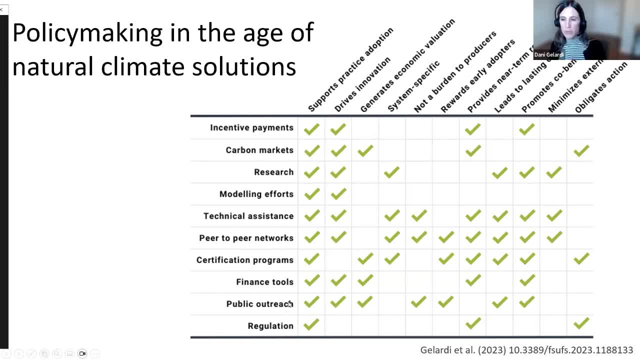 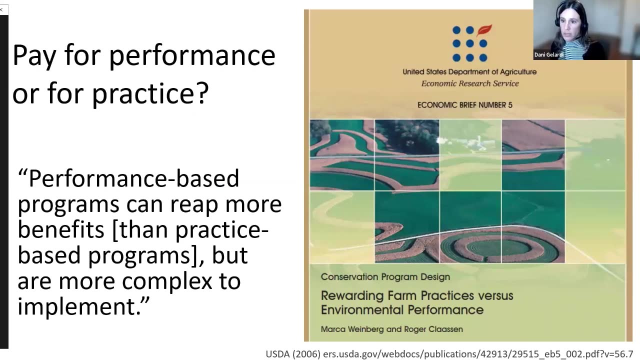 And I don't have time to go over all of these strategies. but because we're talking so much about soil carbon science, I want to highlight one tricky question That comes up when you're building programs to build carbon. When we talk about voluntary and incentive based programming, one of the first questions that arises is: should we pay for performance or should we pay for practices? 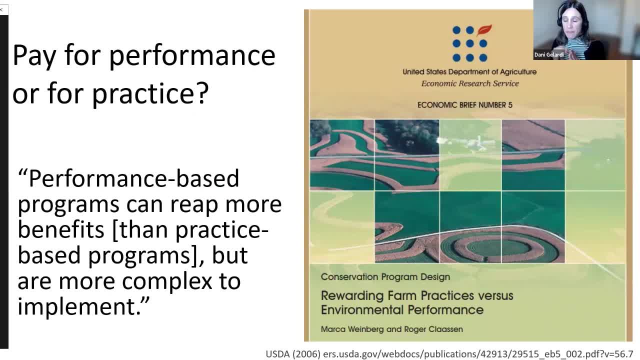 In other words, should a grower be provided with a specific dollar value for every additional molecule of carbon they're able to store, Or should they be provided with a payment to implement a new practice like cover cropping or reducing till, in the hopes that it will sequester carbon, but without the guarantee? 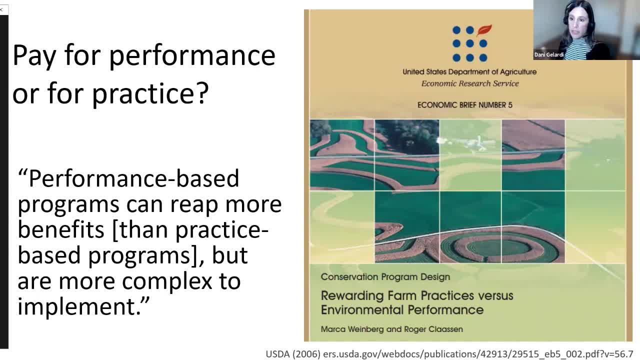 That is a very familiar model from programs like the NRCS, EQIP or, in Washington State, Sustainable Farms and Fields. As early as 2006,, the United States Department of Agriculture conducted an analysis on those two options to find that paying for performance can reap more benefits and actually be more cost effective. 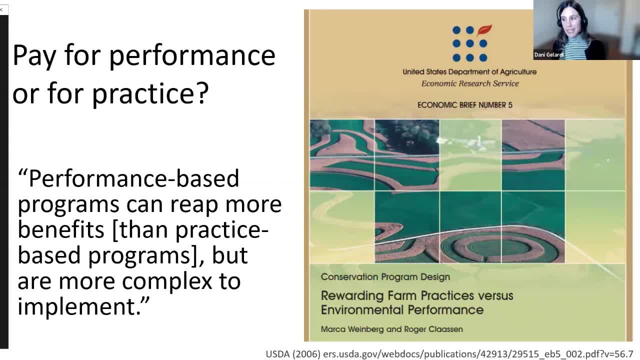 However, they are very complex to implement, And this is unsurprising given all that we know about how hard it is to even measure performance in the soil carbon space. So, because of this, we have tended to lean towards paying for practices, in the hopes that most of them will lead to performance in the form of increased soil carbon. 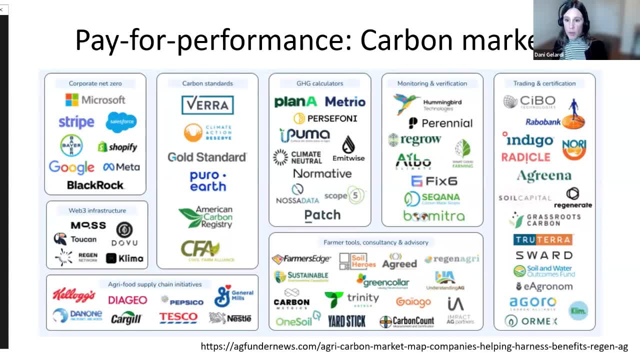 Carbon markets are one strategy that actually does pay for performance by contracting with a grower who agrees to pay for performance. However, there is a lot of attention and funding in the space right now And actually because of that, carbon markets have been a great driver of innovation. We may not have the spectroscopy or remote sensing measurements if we didn't have all of this interest driving quantification of soil carbon. 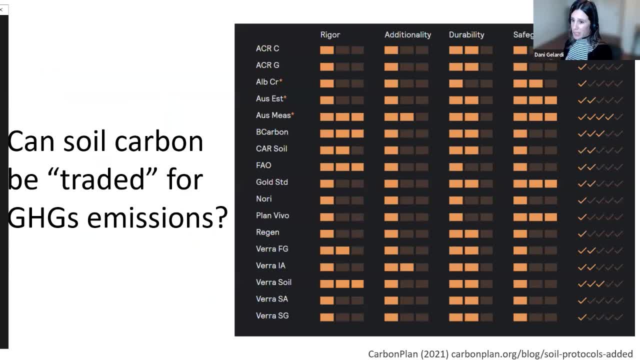 But of course there are major challenges with markets. I won't go over all of the various social aspects of markets, but instead just focus on some of the scientific challenges, As I've described. it's really really hard to know if your practices are going to, or already did, increase soil carbon. 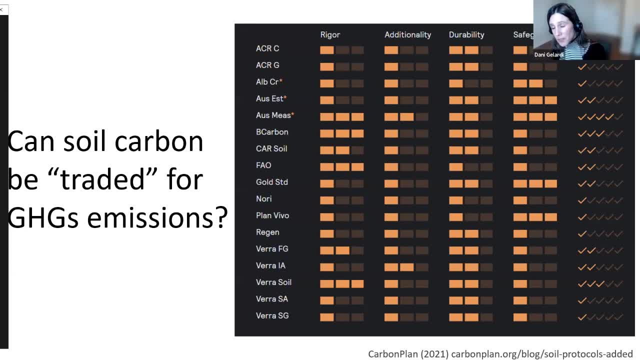 This creates challenges when soil carbon is being used as an offset for other emission sources. For example, if a factory continues to emit greenhouse gases, or maybe even increase greenhouse gases In exchange for paying a farmer to sequester carbon elsewhere, that is not actually guaranteed. 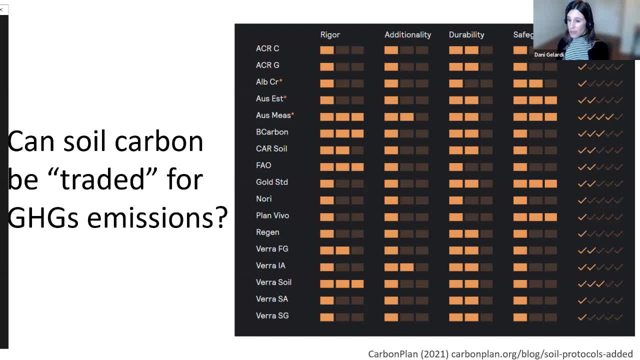 This can lead to a net increase in greenhouse gases or social inequities, by just moving pollution from one neighborhood to another. A group called Carbon Plan recently reviewed the 17 most common soil carbon offset protocols to determine that half of them only scored one out of five in terms of their scientific rigor. 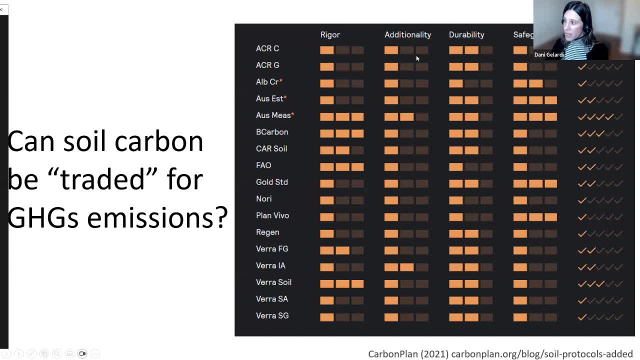 In terms of whether or not that practice would have helped, In terms of whether or not that practice would have helped In terms of the permanence of the soil, carbon and the protection for growers. So this is not a webinar about carbon markets. 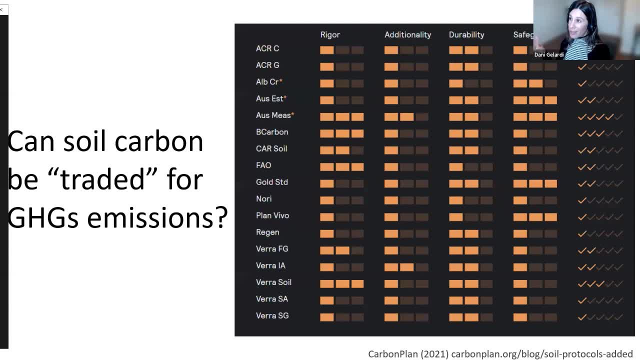 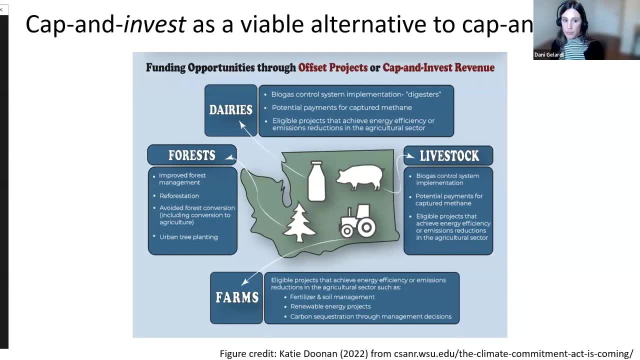 There are a lot of pros and cons, but it is important to note that those challenges in measuring soil carbon or building soil carbon do have real impact on the marketplace. One approach that has been adapted in public markets like those in California and Washington does offer a viable alternative. 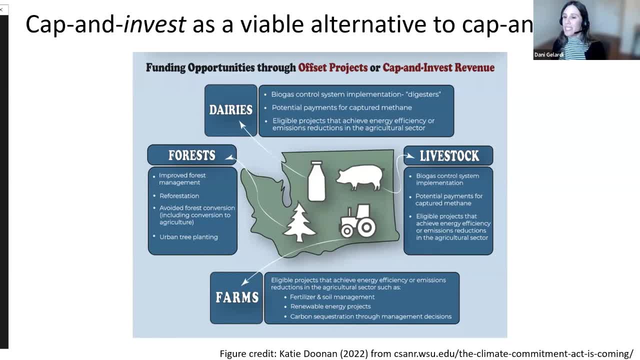 In these markets, soil carbon is not listed as an offset, So you cannot trade your emissions for new farming practices. Instead, these markets sell emission allowances and then take that revenue and invest it elsewhere in projects that can increase soil carbon. This means that soil carbon is not on the hook for mitigating climate change, but is nonetheless very significantly invested in as part of a larger market. 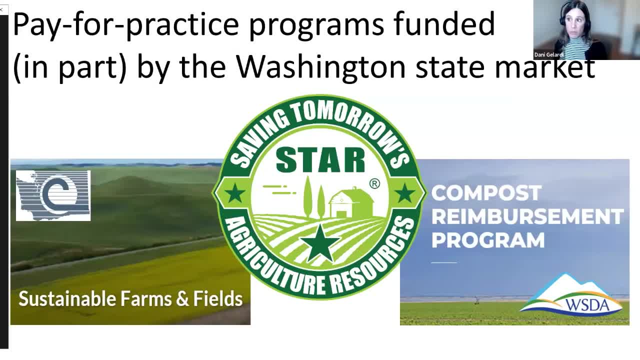 This means that soil carbon is not on the hook for mitigating climate change, but is nonetheless very significantly invested in as part of a larger market. So here in Washington we do have a cap and invest market where soil carbon is not an eligible offset. 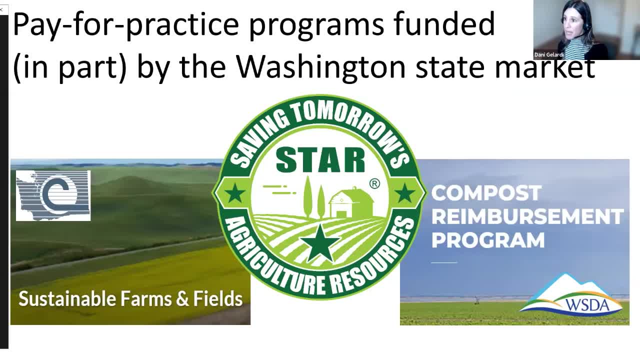 However, the sale of emissions allowances have paid for a lot of pay for practice programs. Some of those that are near and dear to people in this room- sustainable farms and fields- has been partly paid for by the state market. We have a new compost reimbursement program at WSDA. 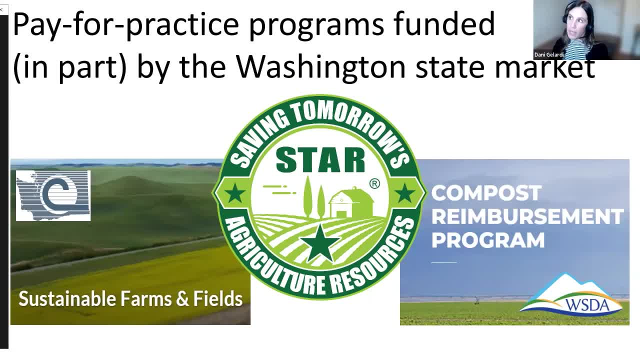 So again, we are paying you to apply compost, We are not paying you to sequester carbon. so practice instead of performance. And a new program coming online called STAR, where it actually started in Illinois but is new to Washington, where you can sort of brag about your conservation practices through. 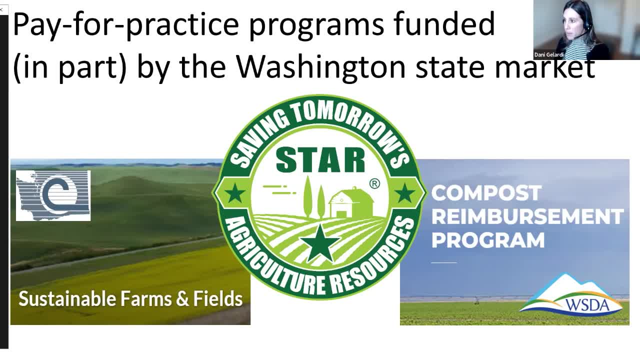 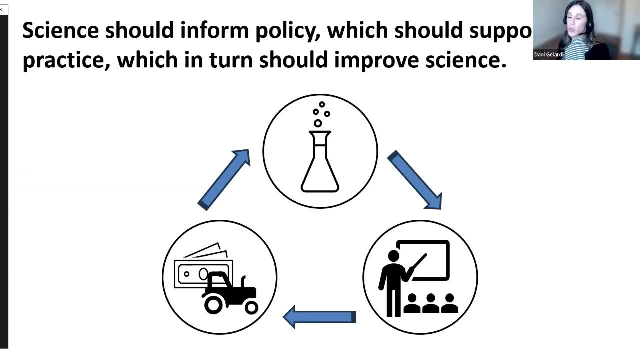 a branding initiative, And these were all invested in by the state market. Because soil carbon is dynamic and complex and encompasses so many scientific, social and economic questions, it really requires a sort of similarly complex and multi-pronged strategy to increase it. So, whether you are paying for practice or paying for performance, 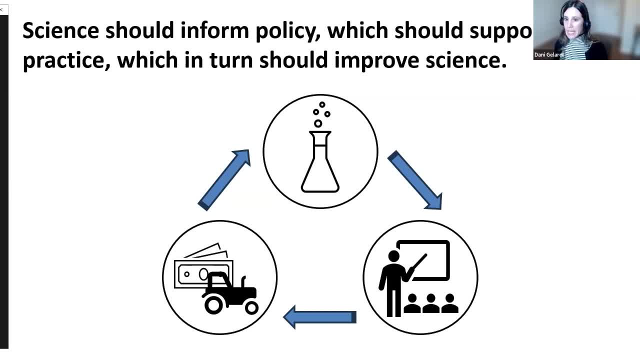 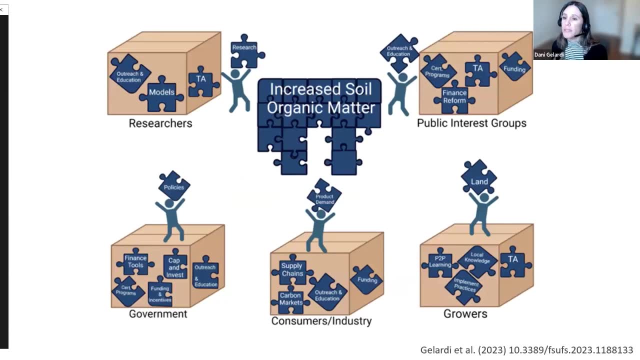 or using models versus using samples. in Washington, we've attempted to build soil carbon within a policy, soil carbon policies within a framework where science informs policy, which supports practice, which in turn should improve science. So having a lot of different stakeholders at the table. 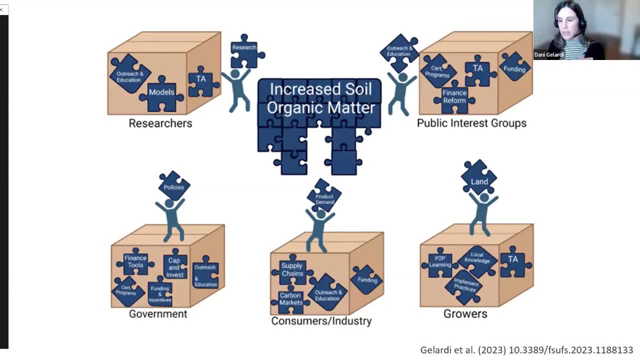 Which, of course, is one of the reasons I'm excited to be invited to talk with the Center for Technical Development today and a lot of technical assistance providers, Because this is an all hands on deck issue. This is more than just climate mitigation and carbon sequestration. 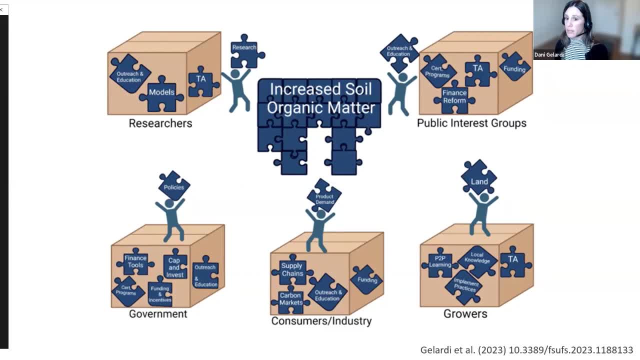 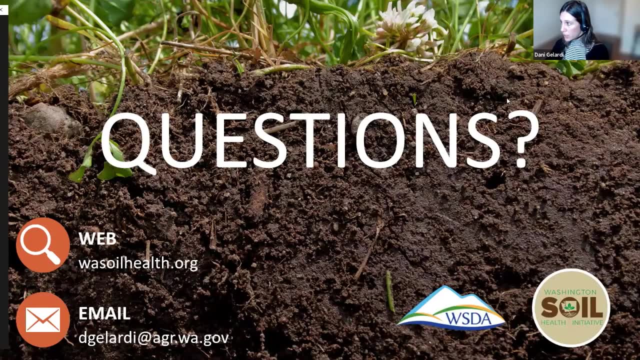 but about preparing societies and growers to be resilient through future climates and helping us all adapt. So a lot of what I've presented here can be found at this QR code in the top right. this is a paper that is mostly about programs and policies, but also kind of covers all of the science. 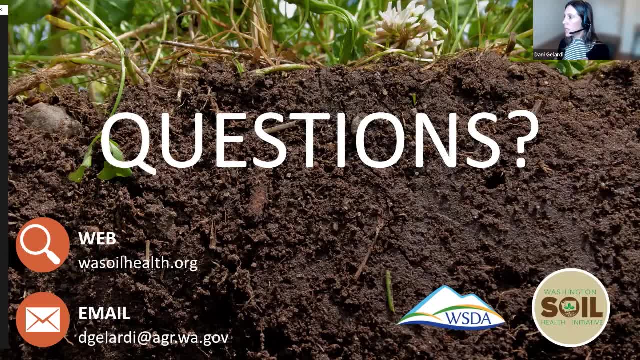 that we talked about, including the measurements and estimation, And with that I will look at the chat, but also anyone, please feel free to ask questions. Who are the PIs at WSU looking at remote sensing techniques? So Kirti Rajagopalan has a grant proposal in right now and does some of this. 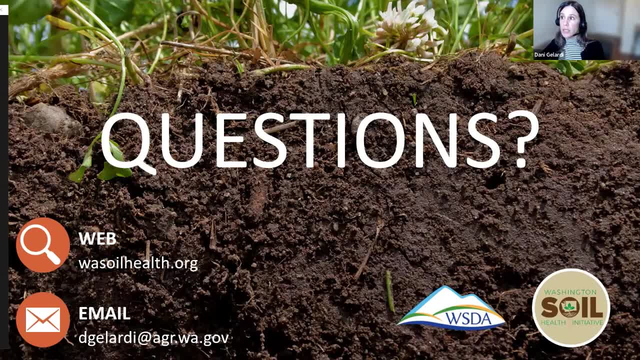 work. already She has been using remote sensing to estimate double cropping and cover cropping in the state, But she also right now is working on remote sensing for soil carbon estimation. So it's Kirti. I'm actually on that project team as well. Georgine Yorgy- There's a lot of people on. 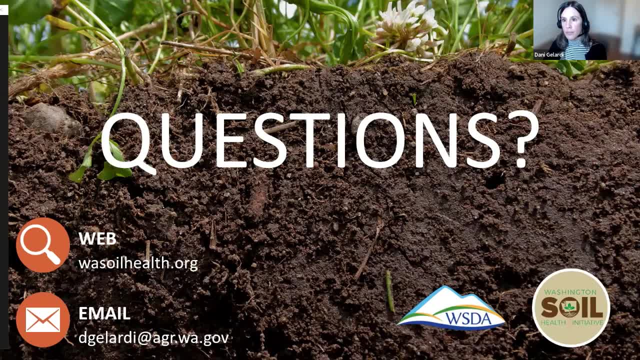 it, but Kirti is the PI And I saw someone link to soil carbon stock monitoring. Thanks so much for that resource. You mentioned up to a 14% seasonal flux in carbon for a test site. What elements would create more or less flux in a field? 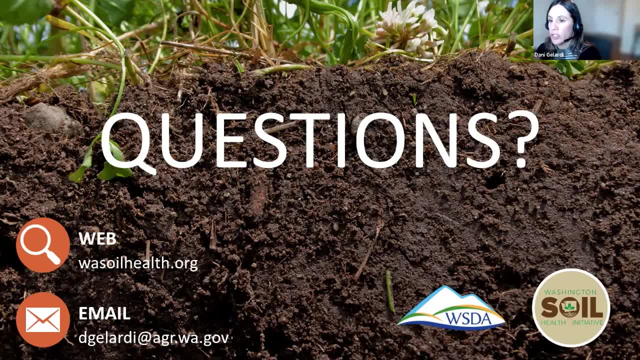 or crop? It's a good question. I can send you a link to the paper that showed the seasonal variation. Some sites were a lot less than 14%. I think it was just up to 14%. But because of seasonal variations plants decompose faster. you know, in wet or warm conditions, things kind of. 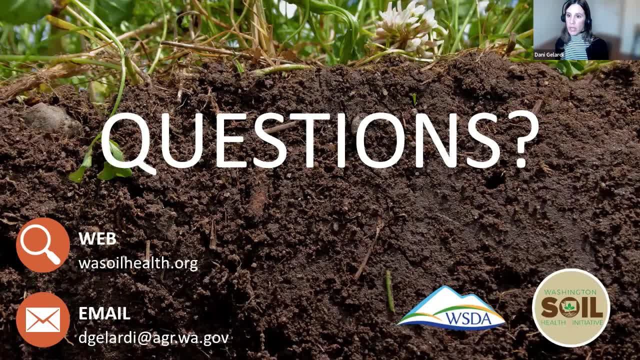 stagnate during the winter, especially on the winter. So I'm going to send you a link to that: The places that they decompose specifically under ice, And so I think a lot of what you see in that seasonal variation is likely just how much of that particular organic matter is quickly decomposing. 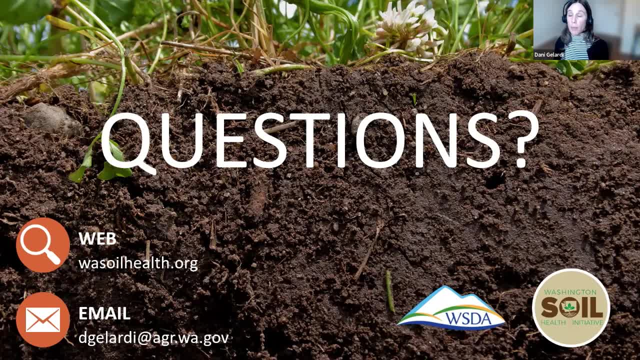 versus times where there is no palm or decomposition has significantly stagnated. but again, that's not my research, So I can send you that paper, Anna, if you want to read more about it. Thank you so much, Danny, and yeah, folks, feel free to just type your questions in the box. 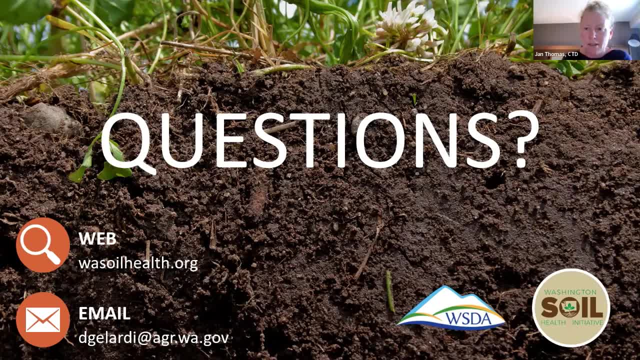 or if that's given you any trouble or you just prefer to ask directly, go ahead and just raise your hand and we can call on you and you can unmute and ask directly as well. I am going to pop the link for the CTD website in the chat as well, and that. 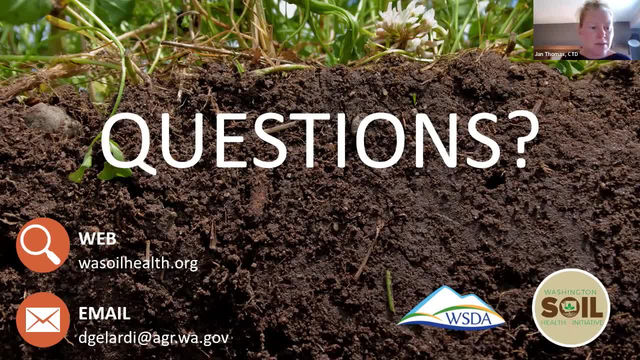 will be where you can find the recording for this a little bit later. No worries, if there are no other questions. um, Anna, while I'm I have you here. I'm going to pull up that resource and drop it in the chat so you don't have to reach out later. 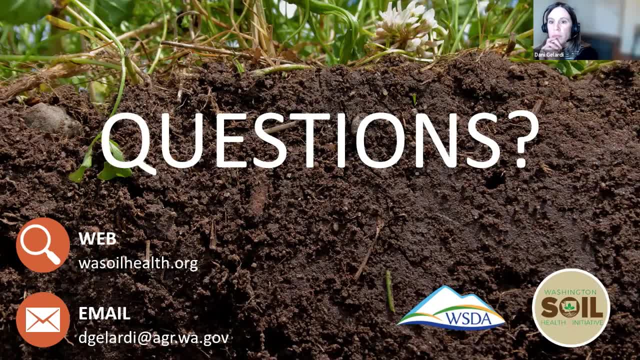 Thank you. Oh yeah, Karen, thanks for plugging the Washg or Washington Soil Health Initiative Newsletter. We have lots of talks, lots of people working on lots of things, so go to washwasoilhealthorg to sign up for our newsletter. John asked: do you think there are any gaps in the laboratory? if we are there on the ground doing the field work and we are trying to 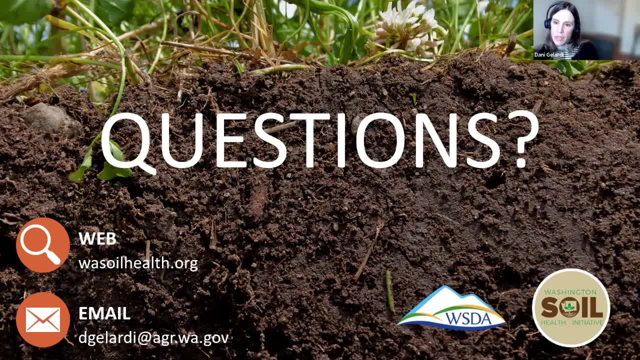 equipment techniques for better accounting for carbon in its various forms in soils. So I think there are gaps. This is also a topic for a whole webinar. But in Washington we have a program called State of the Soils Assessment, So we've taken something like 900 samples in different 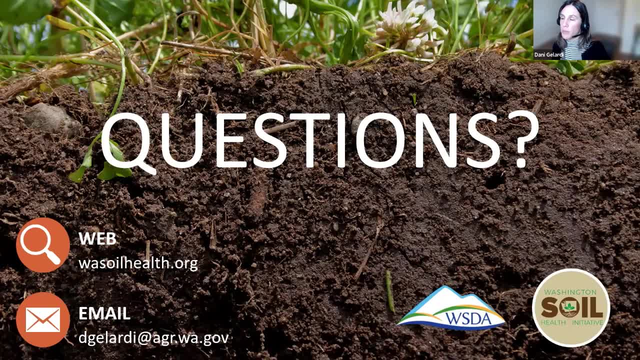 fields across the state. We work closely with WSU on this project And we've been really excited to try to link these different carbon measurements to different management techniques. That is still underway. But one thing we found is that the lab that we have sent samples out to is as variable. 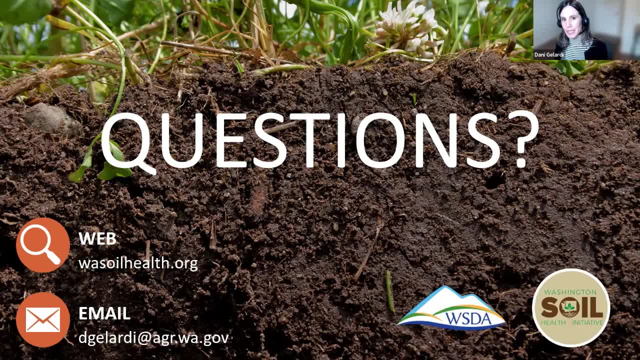 as the soil texture or the management. Even when labs are using the same standard operating procedure, they frequently have different equipment and so need to edit those SOPs first. So we've been working closely with WSU on this And we've been working closely with 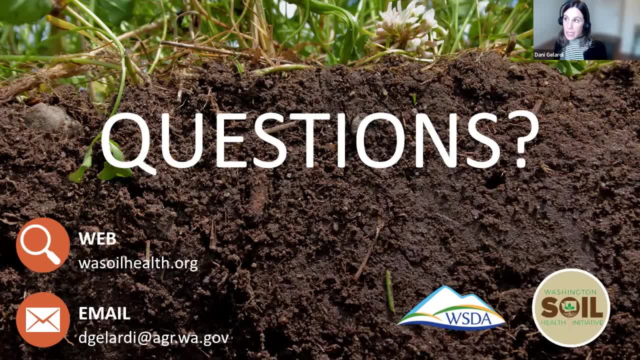 WSU on this And we've been working closely with WSU on this, And we've been working closely with their own use And sometimes they are interpreting things totally different: Different ratios of sample to extractant or different incubation times based on how long their incubators can. 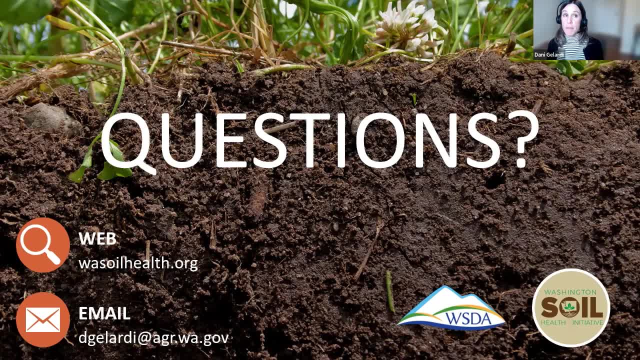 hold samples because of the high throughput. So for me, one of the first gaps I think that could really be addressed is just more standardization of these newer methods. like standardizing methods is a gap that needs to be addressed And hopefully through our project. 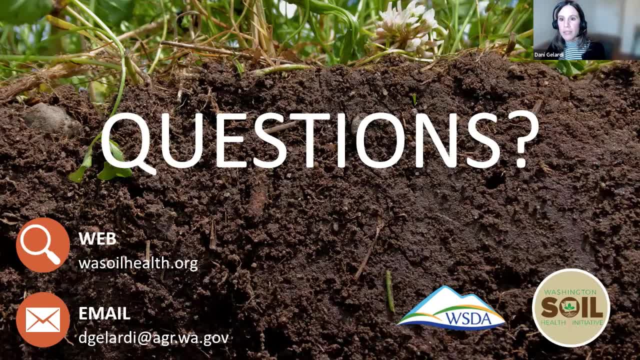 we're helping with that, Dr. Yeah, Surendra just sent. Dr Singh just sent another from the same group on the variation in soil organic carbon. So I will send that to everyone. Thank you so much, Dr Singh. 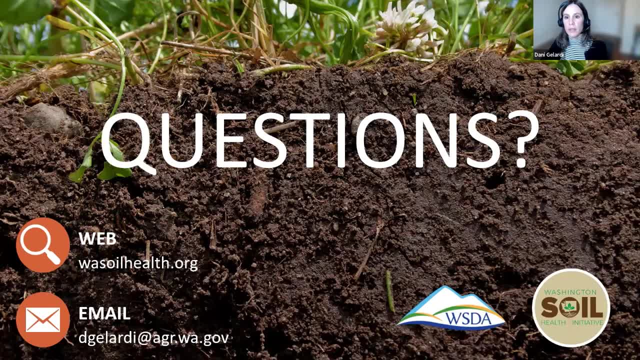 Dr. Yeah, Jonathan, thanks so much for your time. I appreciate it. Dr. Thanks for that. I agree, It's, it's. you know soil, organic matter is not always the most descriptive measurement, but at least you know there's really only two methods out there, which.